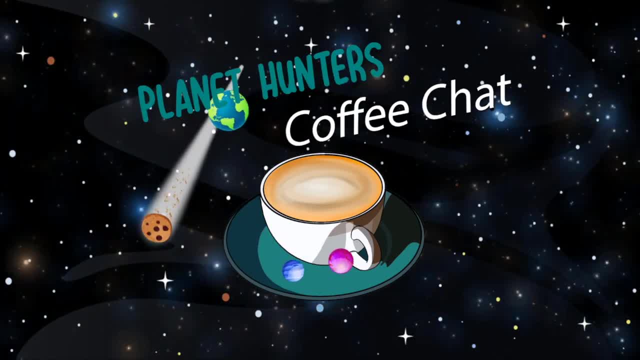 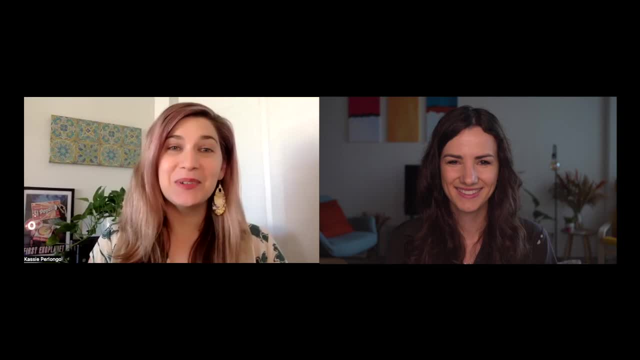 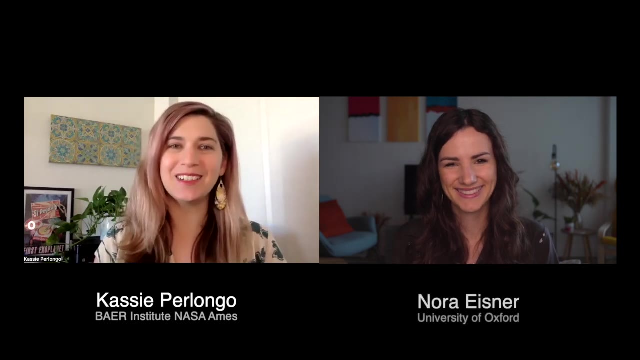 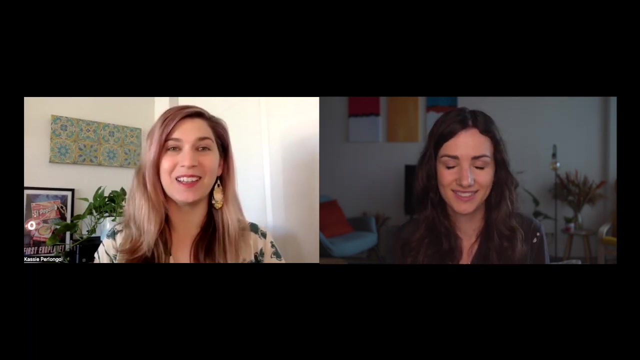 Welcome back to another episode of Planet Hunter's Coffee Chat. I'm your host Cassie Prolongo and of course joining me as always the lovely Nora Eisner. Good to see you Nora. Good to see you too. It's been so long. It has been way too long. Oh my gosh. We were off air so to speak for a while. Do you want to tell them why we were off air Nora? Yes I had a bit of a busy couple of months. I was just finishing my thesis so I handed in a couple of weeks ago. So glad. So glad it's done. And yeah so I was just busy doing that. So I had to write 250 pages about everything I've done in the last three years and I did it. I submitted it and now I have a couple of weeks to rest until I have to prepare for my defense. So I still have to orally defend all the work I've done. So fingers crossed. Yeah congratulations. Well done. 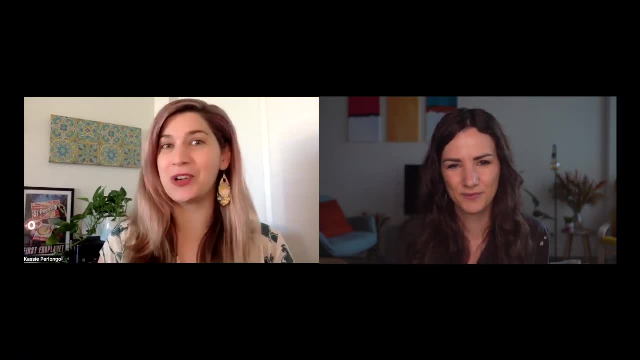 Super proud of you and it's going to be awesome calling you Dr. Eisner pretty soon as well. That's going to be a lot of fun. It hasn't quite sunk in yet. We'll see. Maybe once I actually am Dr. I'll sink in that that's what's happening. Yeah it's going to be great. So we're 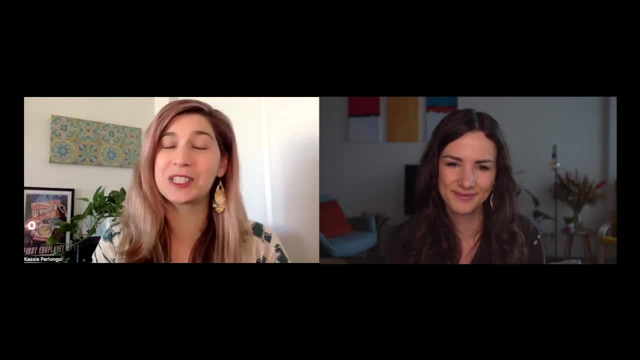 going to have a lovely couple of people who actually reached out to us and asked if what's going on. Are we coming back? And we are back. So we are filming a couple of exciting episodes over the next few weeks and then we might have another break depending on what happens with Nora's defense as she just mentioned. But other than that yeah things are going well. So thank 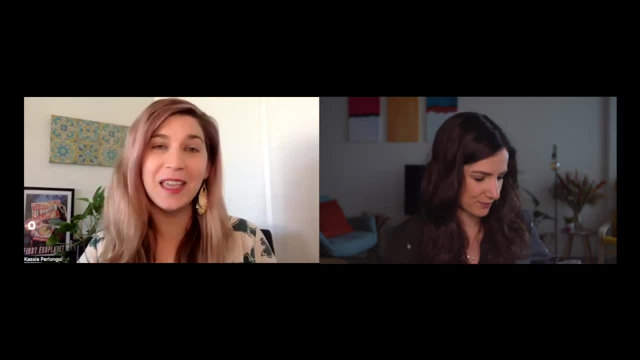 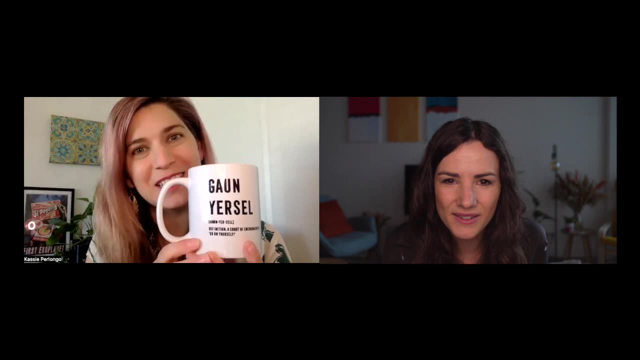 you for joining us today. I hope you have your coffee or tea or beverage of your choice. I have my lovely funny coffee mug today that was given us given this to me. 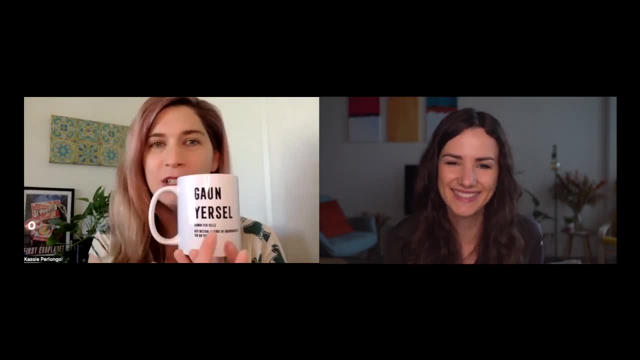 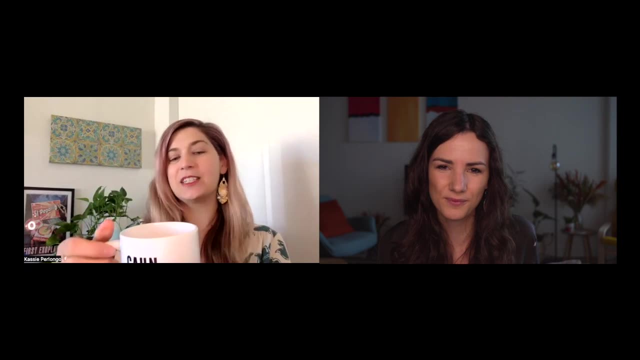 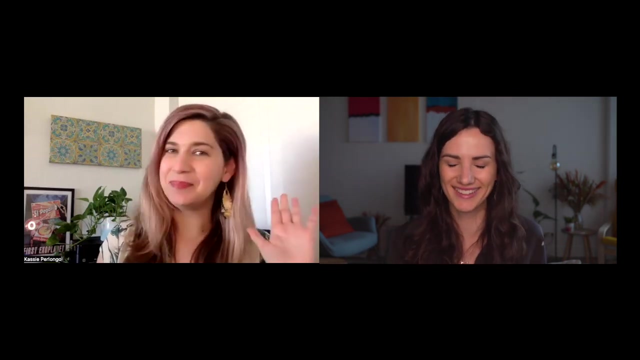 From Katrina who's our social media person. It says go on yourself in Scottish I'm assuming. So yeah she's absolutely lovely and but yeah that says definition a shout of encouragement go on yourself. Go on yourself. Can be on my show for today. I think that's great. Go on yourself. Yeah it's like she said it's like the definition it's like an American saying you go girl kind of thing. Oh okay love it. Love it. Very cool. Go on yourself. Yeah exactly. 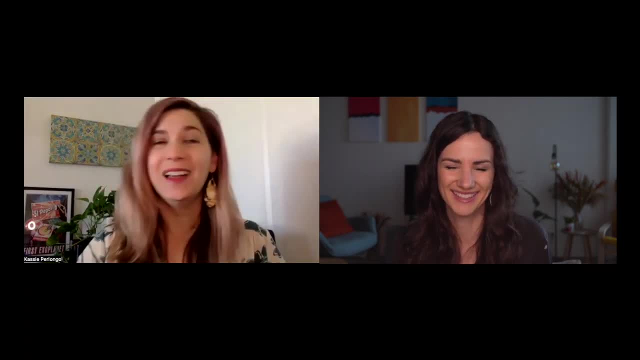 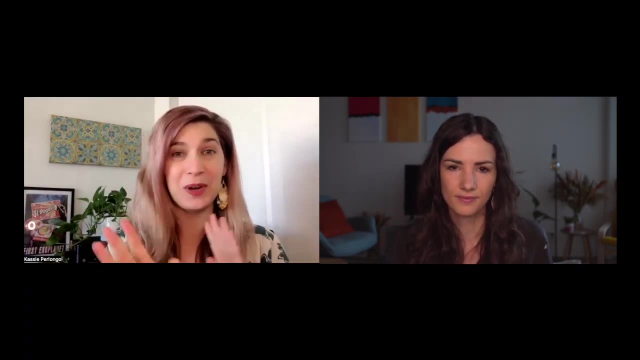 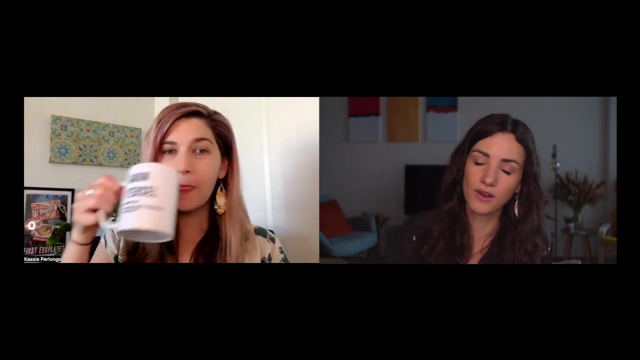 So anyway sorry we're goofy today. It's been a while since we've seen each other. So Nora what are we diving into today since it's been a little bit of time between our last episode and today? So today we're going to look at something we've talked about a couple of times come up there's come up quite a few times actually which is radial velocity observations. 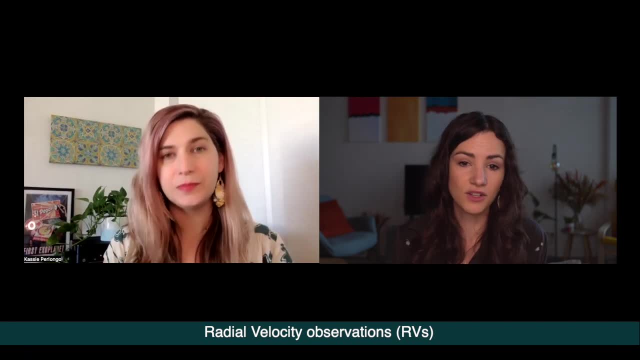 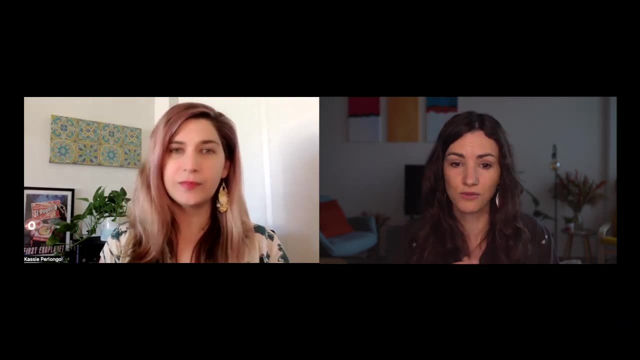 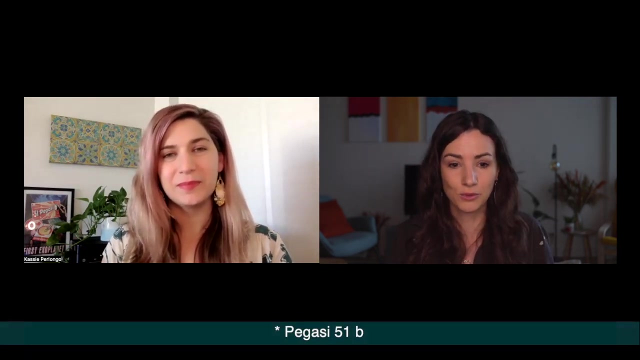 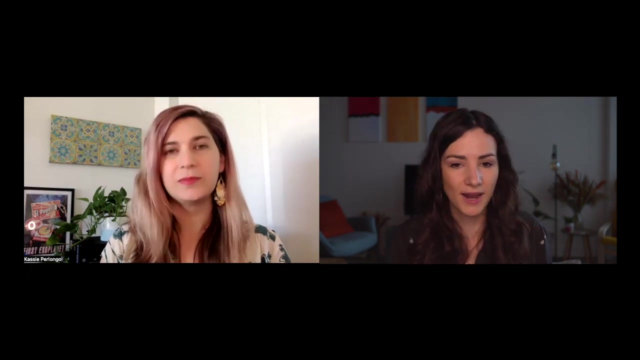 Yes. So this is how radial velocity observations is another technique. to discover exoplanets. It was actually how the first ever exoplanet was discovered, Pegasus 51b, was found with this radial velocity observation or method. But it's now become more commonly used to observe planets that are already known. So already if you found a planet using the transit method then often it is observed using the radial velocity method because it can be used to determine its mass. And the reason why determining the mass of a planet is so important is because if you have the radius of the planet, so kind of how big it is, and you have how heavy it is, then you can determine roughly how dense it is. And this density can give you an insight into what it's made of, whether it's a rocky planet or whether it's a gas planet, which is exciting because if we're looking at these planets that's something we want to know. And the mass can also help you determine whether it has a large atmosphere and just give you much, information than we would otherwise have just from from observing transits and from having the radius of the planet from um that method so we mentioned the radial velocity method um like i 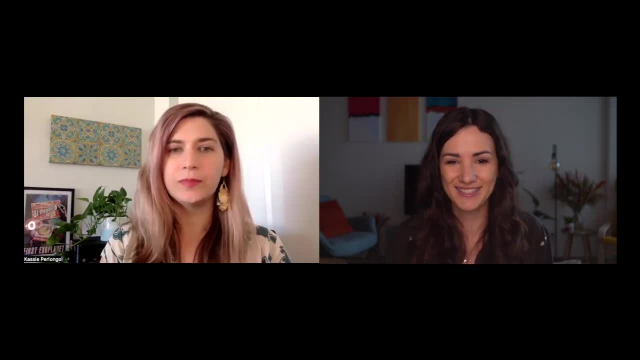 said in quite a few episodes i think the last time we mentioned it this could be wrong but i think the 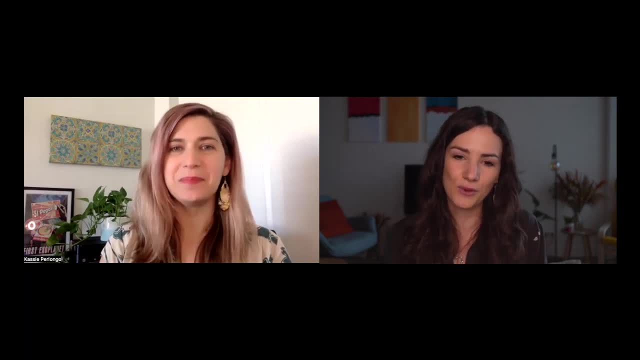 last time we mentioned it is when we talked about the triple star system so yeah is that right um 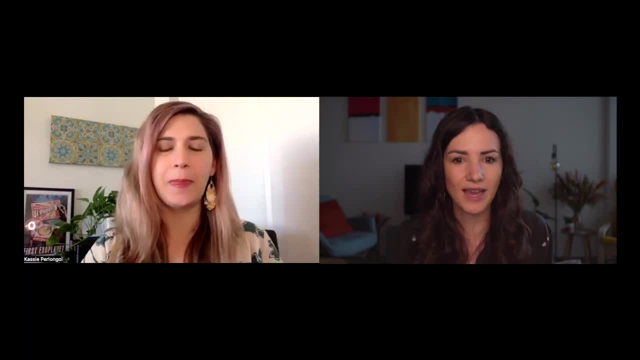 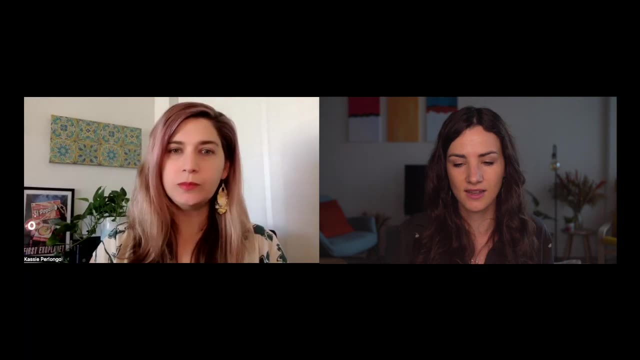 i think so too yeah i think the um yeah we talked about it then so that just shows the radial velocity method is useful to to look at both planets but also to look at stars so i think we 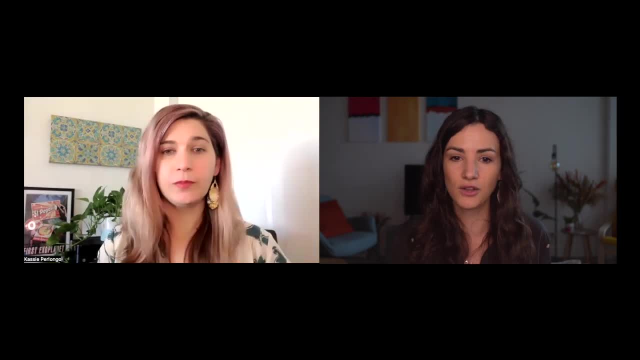 should briefly go over what what it is and then we'll look at some code and we'll look at some data afterwards how does that sound that sounds great let's dive into it and i'm pretty sure we've 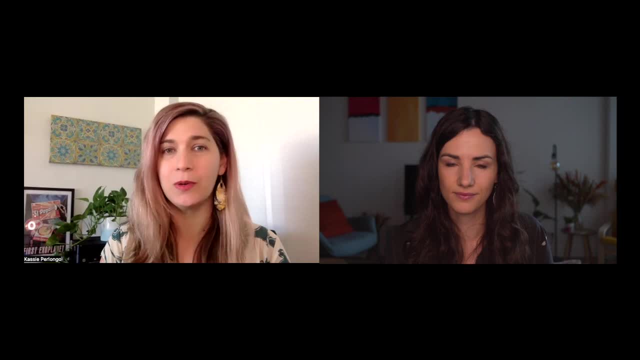 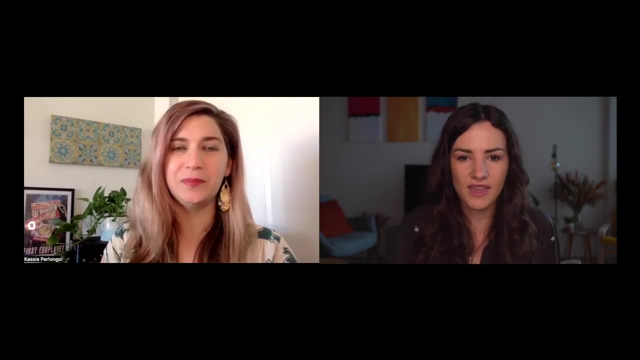 had some comments about this on our youtube as well so hope that you guys get a lot of out of it so let's dive into it nora that sounds great cool um okay yeah so the radial velocity method 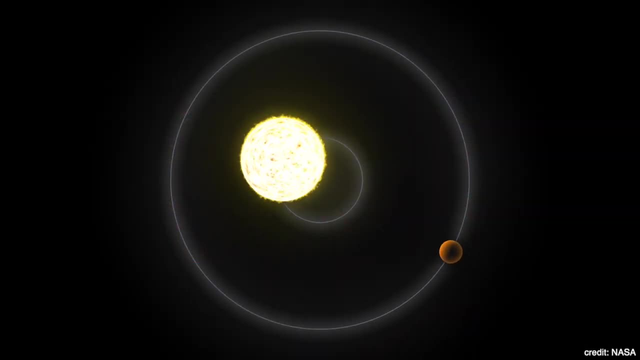 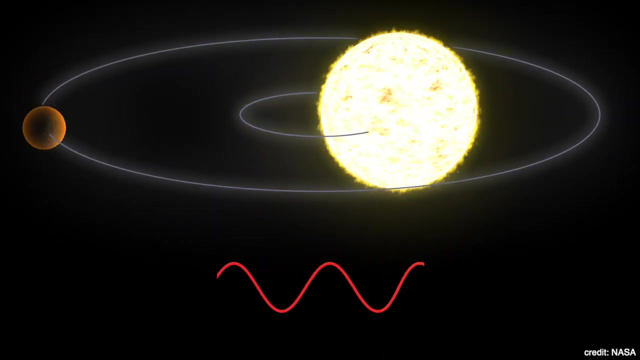 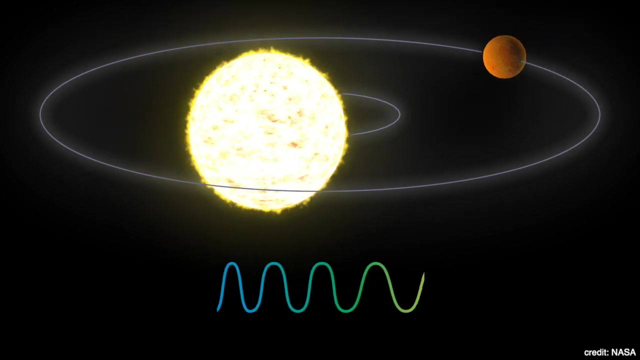 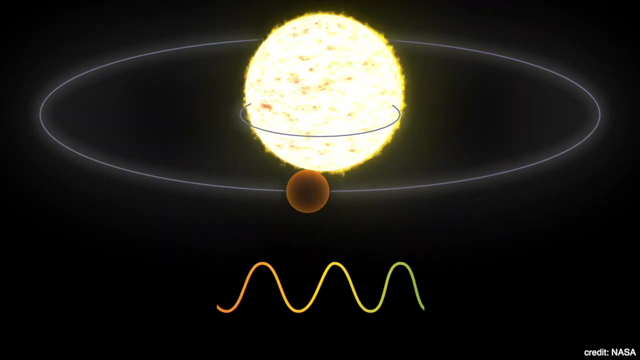 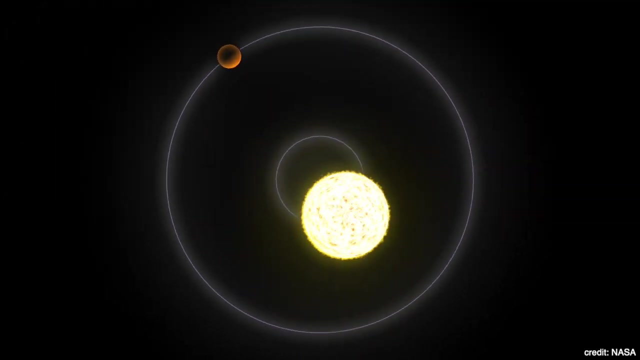 is if you imagine a planet's orbit around stars um they do a nice circle around these stars um what's probably slightly less well known is that the stars also orbit around the planets so they also orbit well they both say they both orbit around a common center of mass around a common point uh which is very close to the star so the planet does a big circle and the star does a tiny tiny little wobble um on on its orbit it's also a tiny little circle but because that that star is also wobbling around the planets it's also orbiting around the planets so it's like a little bit of a rolling caused by the gravity of of the planet that's going around it 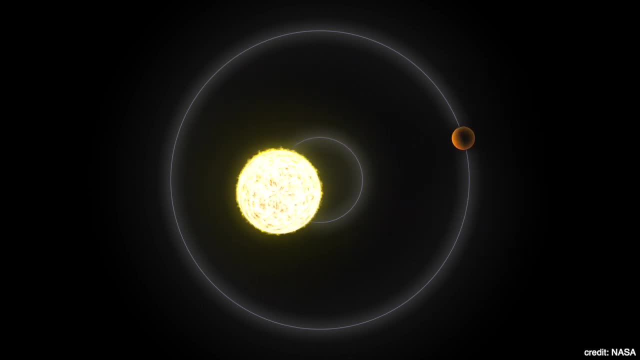 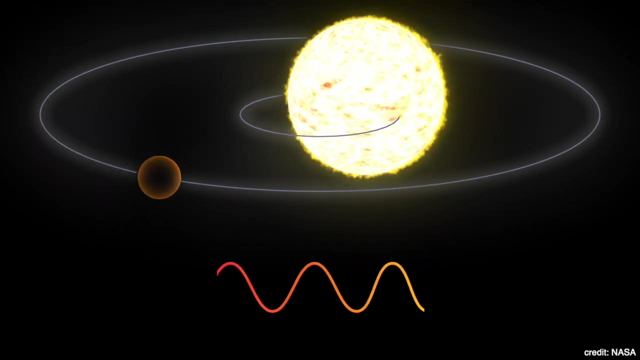 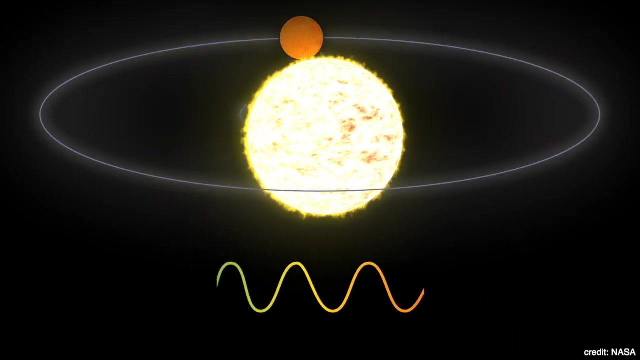 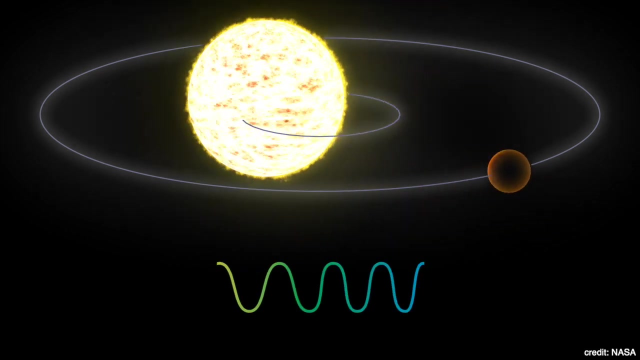 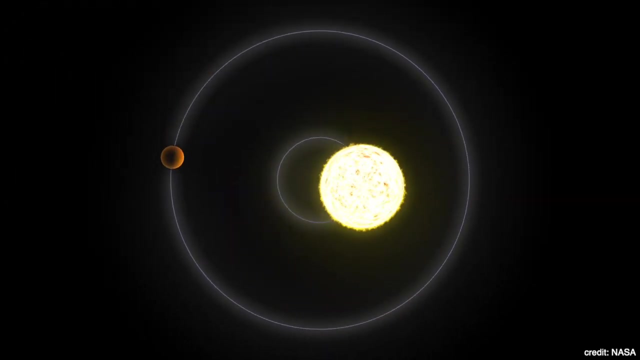 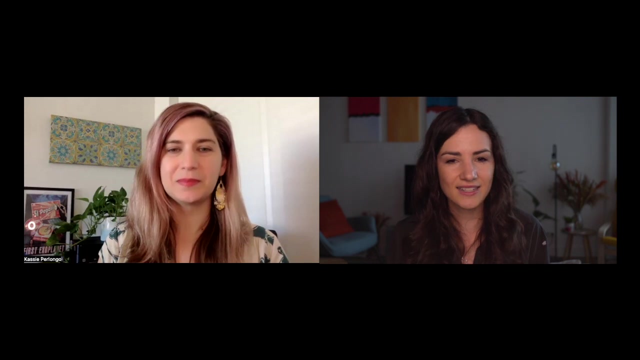 that means that that star is sometimes moving towards you and it's sometimes moving away from you because it's moving in that small circle very very tiny um so if we're looking at the light of the star that light is sometimes kind of as the planet is moving to sorry as the star is moving towards you that light is more squished together so it appears more blue and if if the star is moving away from you that light is stretched out and appears more red right so this is called the doppler effect um if we measure the light we can see it sometimes a bit more red sometimes a little bit more blue it's analogous to um you can have this with sound as well so sound is also waves 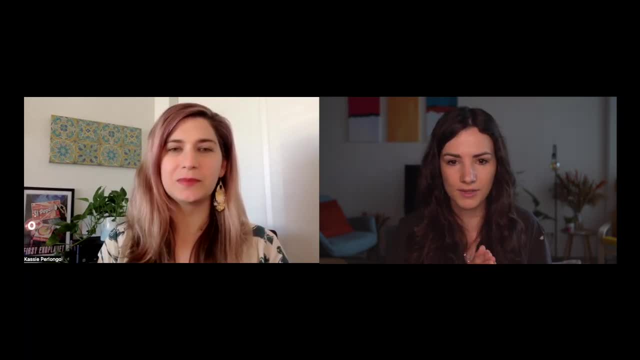 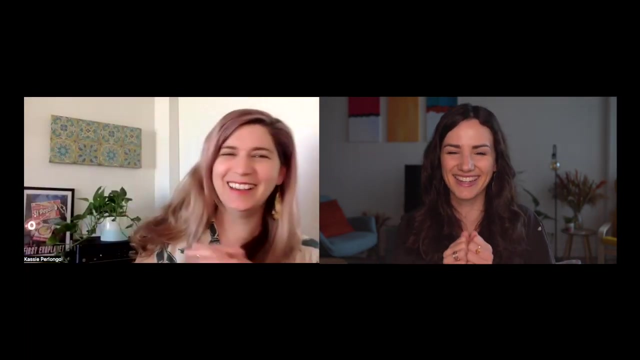 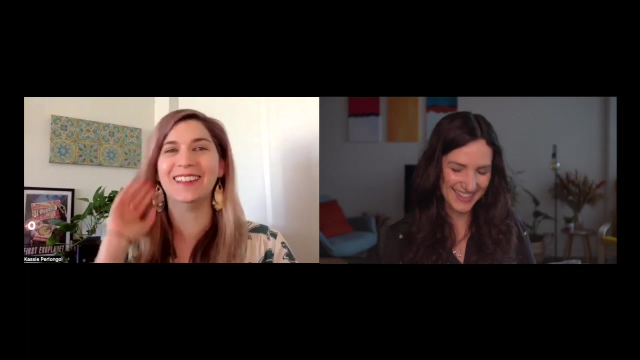 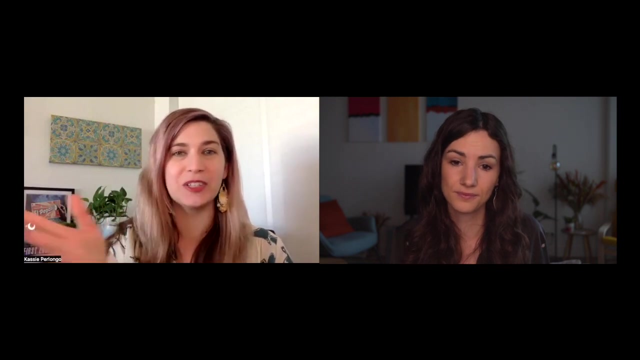 um and if you hear for example um an ambulance moving from yeah you you might have heard this already um if you have an ambulance moving past you the sound will change from as a if it's moving towards you or away from you cassie why don't you why don't you give us a little illustration of what that would sound like that was great off the cuff i'm sorry that was good this is why you keep me around nora oh my god the sound effects yes but that's you hear it all the time police sirens fire engines or an 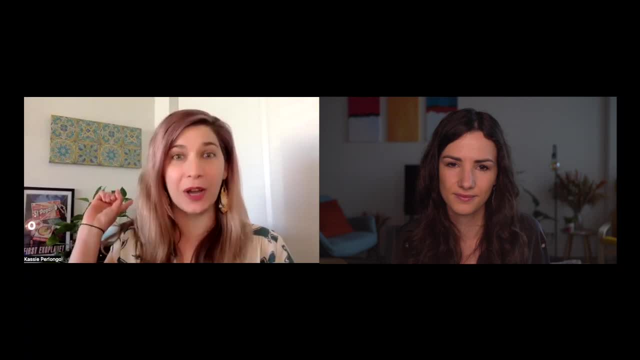 ambulance yeah exactly and you're like oh gosh you can hear it coming and then it's like oh my god when it's there and then when it goes away so the same same kind of effect so that's the doppler 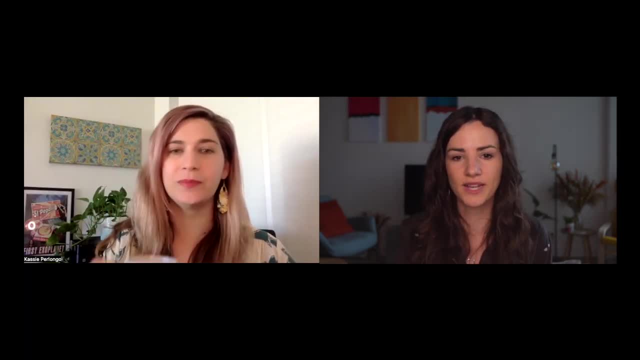 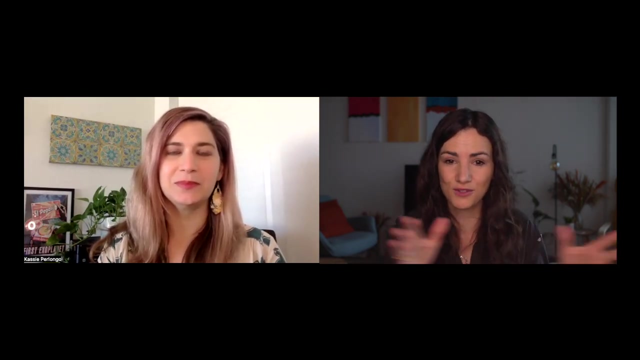 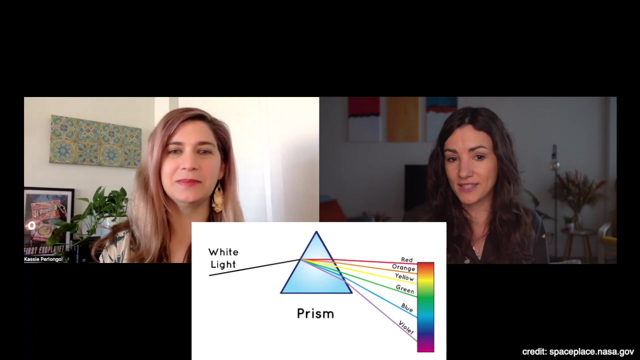 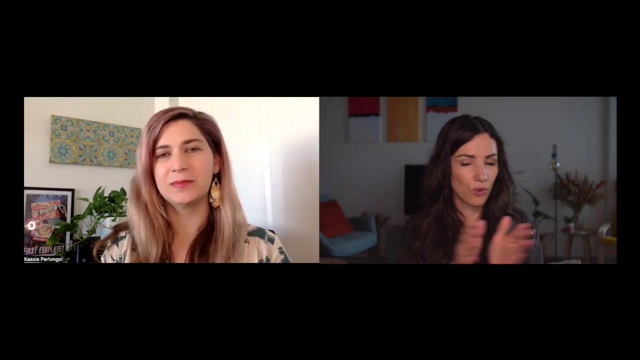 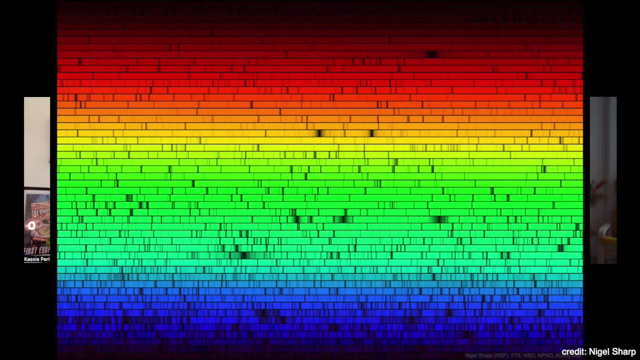 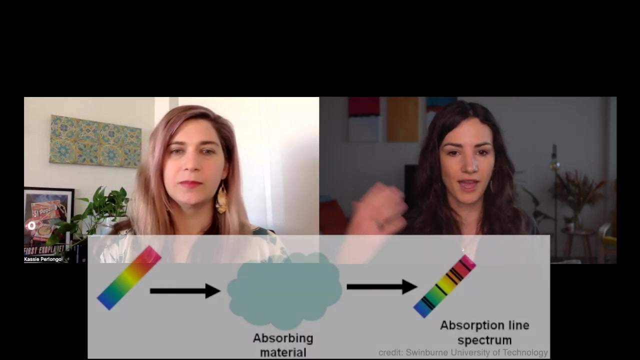 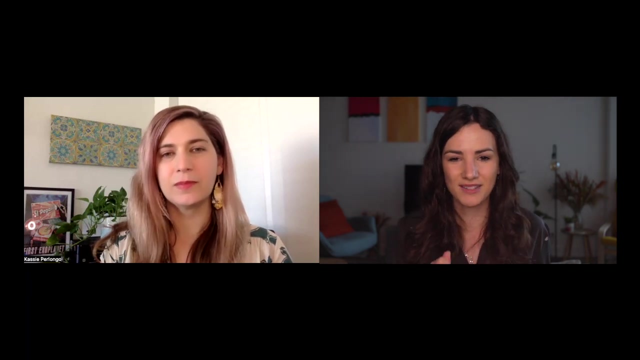 effect for sound as you mentioned yeah exactly so we're just looking for this doppler effect not in sound but in light um so the way we do this is if we take the light from a star um light is made up not just of one wavelength it's made up of lots of different parts so if you think of light passing through a prism you might have seen that or um light reflecting off a cd you also see a pretty little rainbow um because that light is is splitting is being split into all of its different parts all the colors of the rainbow so if we do this to the light of the star we can spread it all out we see all of the different colors and there'll be certain parts that are dark so there'll be certain parts that have parts of the light of this it's called a spectrum certain parts of the spectrum that have been blocked out so it's being blocked out because the light is passing through the atmosphere of the star um which is causing the light to spread all the way over this wavy girl we call them absorption lines so where it's spread lying that the light is going to be going to go to is a place called white light so treat it as if it was twilight it's getting to the plus directions we call these we call them absorption lines so where the light has been absorbed by the atmosphere so if we we 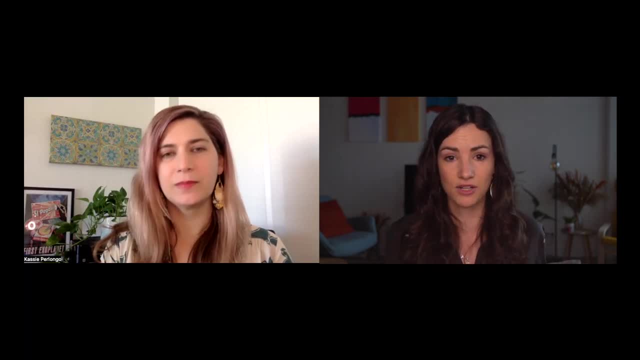 can take these we will see an example of this in just a moment because we'll show our spectrum 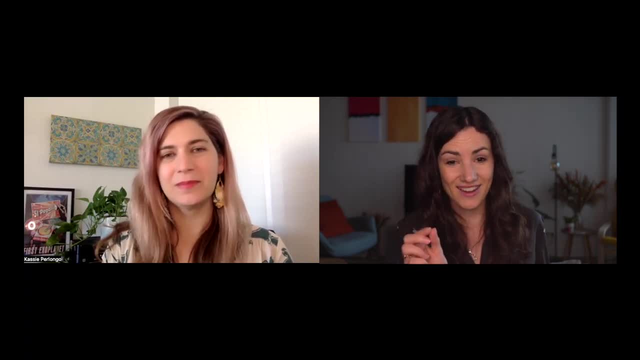 we can measure the location of these lines really really carefully and those lines will shift either of the star which is induced by the planet going around it so that can tell us about the existence of a planet there or it can tell us about how big that planet is so if you have a large planet that's close to the star you have a really big wobble of the uh of the star and if you have a small planet 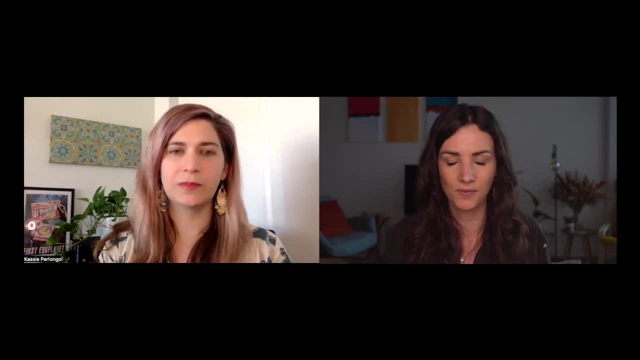 that's far away you have a much smaller wobble of that star so that can knowing those properties can tell you about um what planet we have and what its properties are slight sidebar will the 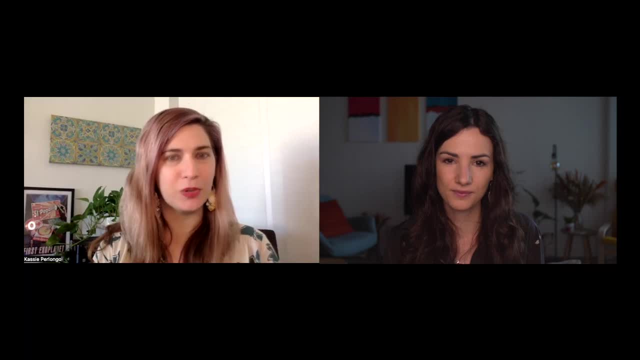 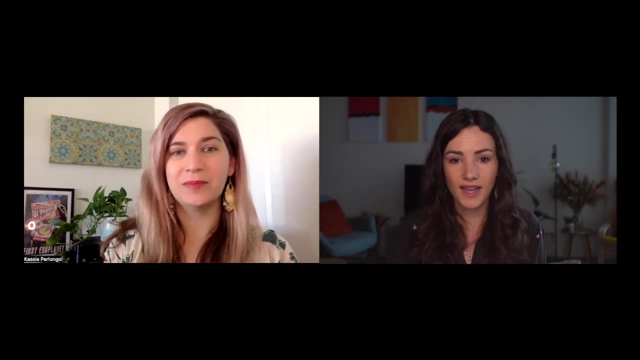 james webb telescope be able to measure things like this a little bit more succinctly or more efficiently or yeah uh yeah yeah uh the james webb can definitely do this um it's got a spectrograph 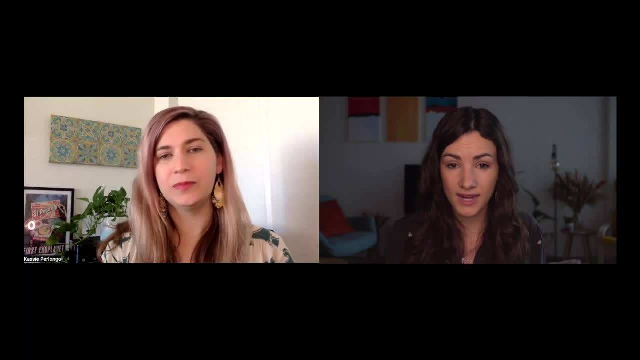 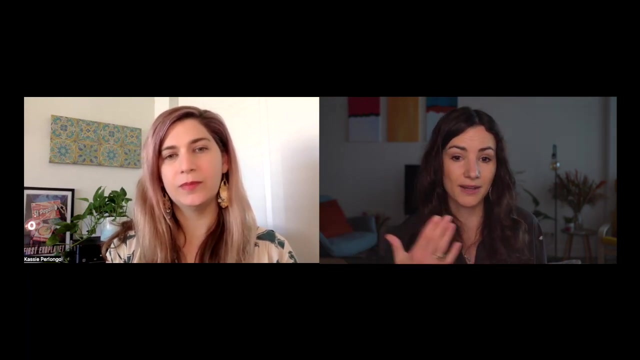 on board um what the james webb will be really good at is doing um also taking these spectra so also taking the light and splitting up into lots of different parts and then instead of doing this over time to kind of get the wobble doing this the um planet passes in front of the star and if the planet is passing in front of the star 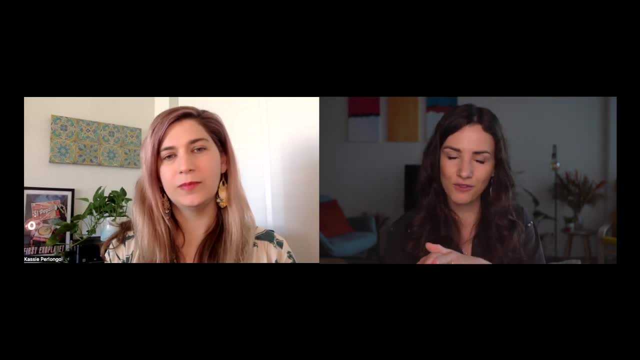 then part of that light from the star will pass through the atmosphere of that planet which means we can kind of determine which sorry so which lines are dark so these absorption lines 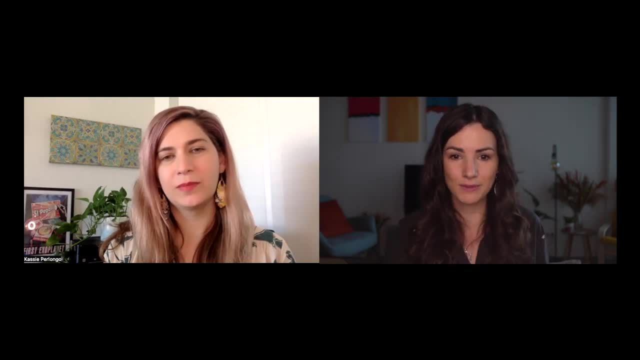 tell us what's in the atmosphere so this can tell us about what's in the atmosphere of these planets and these tools on jwst will be really good for that so that's really exciting that is really exciting and we'll be able to know if these are 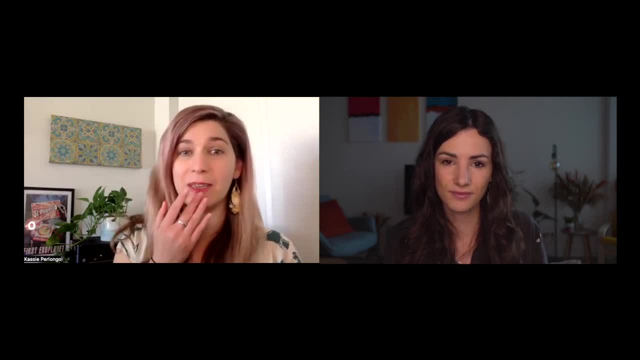 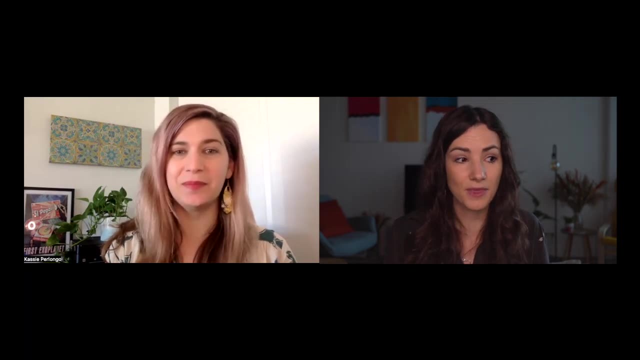 potential habitable um habitable planets or not maybe depending on its atmosphere or rocky yeah a lot of a lot of different things going to habitable zones yeah um but they might be able to tell us whether there's water in the atmosphere or whatever else is in the atmosphere sorry for 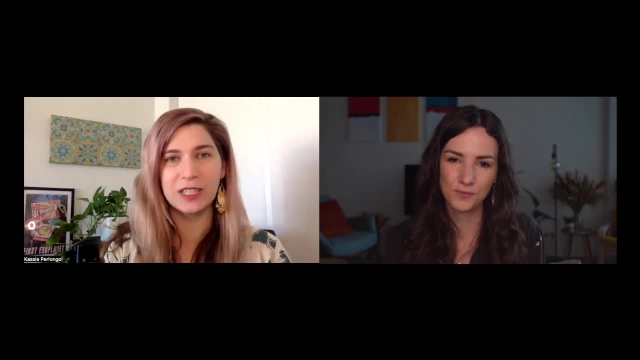 the sidebar thank you very much for answering my question excellent okay so let's look at these uh absorption lines that you mentioned as well yes okay i'll show my screen 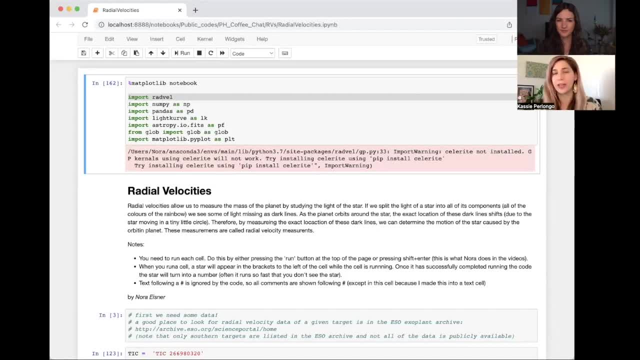 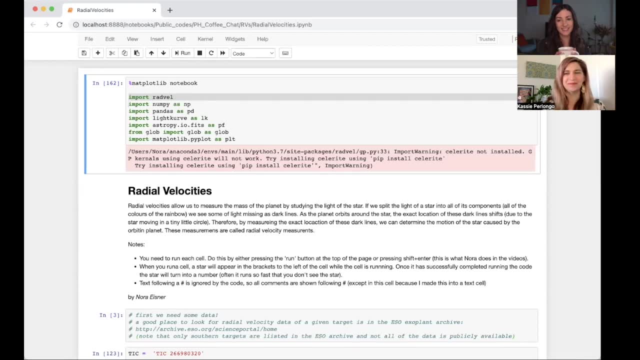 oh my gosh i'm drinking cold brew today and let me tell you that is the best thing to have on a monday morning i am it's in a team up but i'm actually drinking water today i'm cheating you are it's okay it's okay we won't judge you i had a lot of coffee when i was writing my thesis i'm trying to 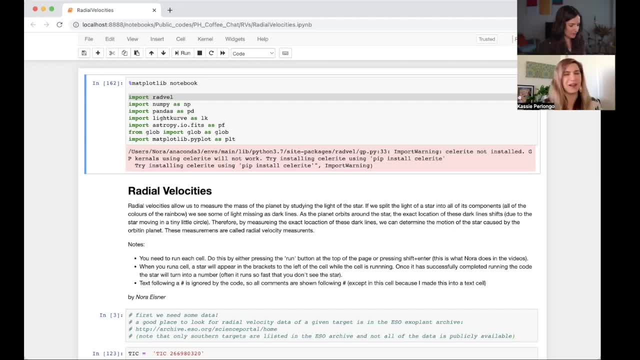 turn it down smart come down from the caffeine high okay gosh all right so this is cool so we've got a new notebook i'm sure everyone will be really excited about this yeah so um i prepared a notebook i won't code live i did this right at the beginning and i haven't 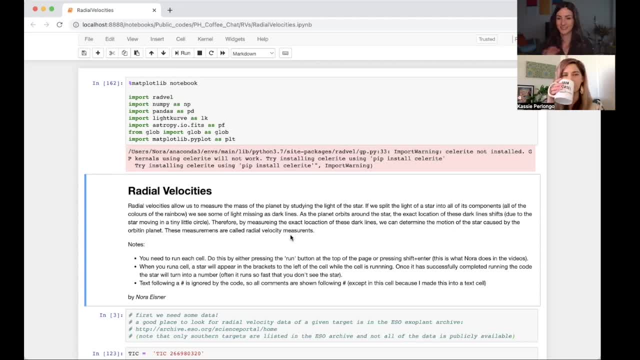 done it since because i made so many typos that actually i was i decided to stay clear um but we 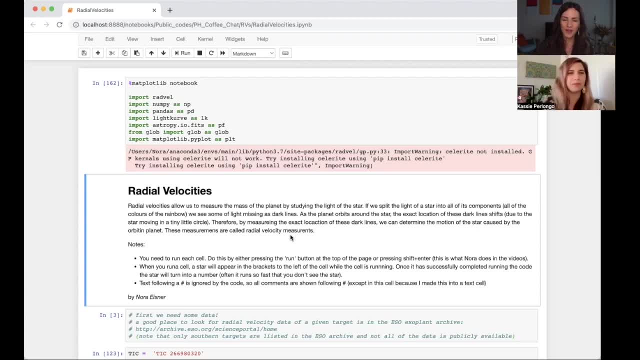 could go back to that um anyway so um radial velocity data is taken by lots of different telescopes from all over the world most the time the data isn't publicly available but there are certain data sets that are publicly available so we'll be using one of those data sets today and the place where we can get those before we even go into what the data is is on the eso um archive 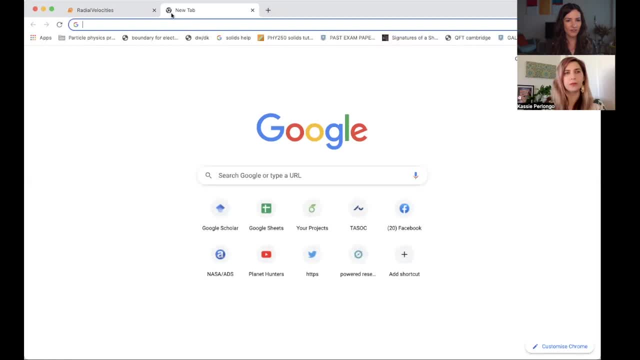 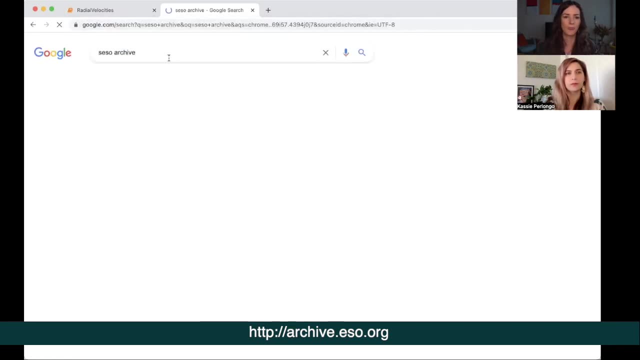 so the european southern observatory archive we have very we have previously mentioned this i think oops we'll just google eso archive that's it this is why i didn't i don't type live anymore um 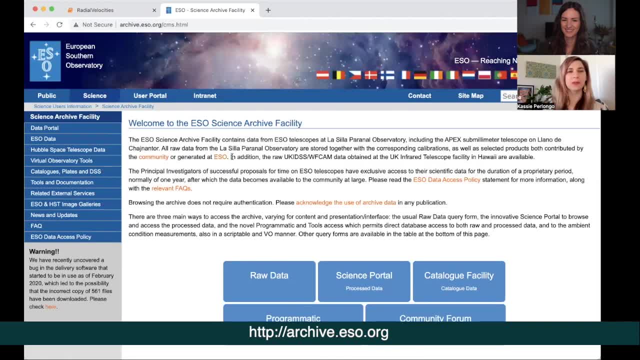 it's like me when i'm trying to back into a parking space and i see people staring at me and i go over the lines 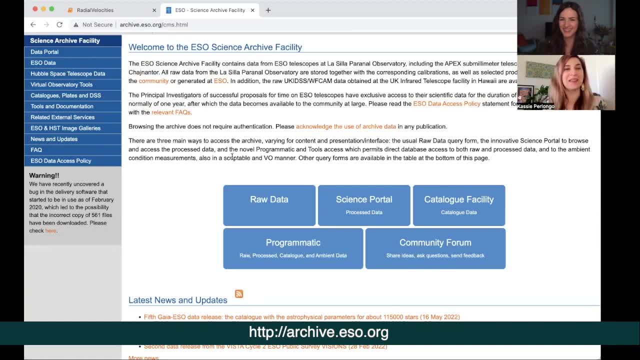 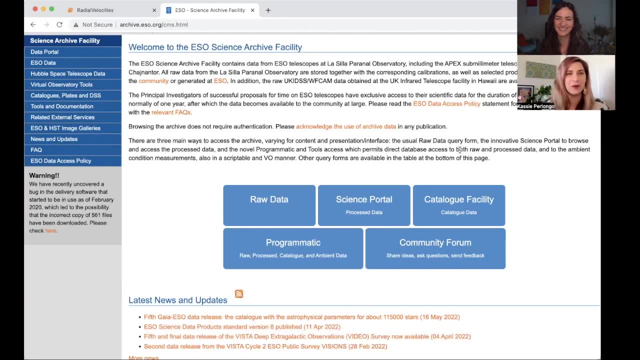 when i back into a part because it's the anyway sorry the same kind of thing don't look don't look while i'm back into a parking space anyway sorry second sidebar for today back to eso 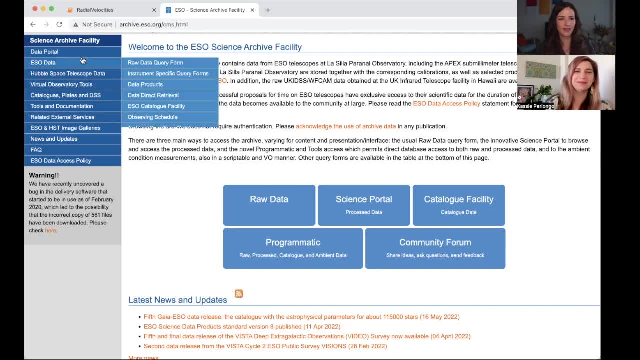 the science archive facility yes so we can i'm going to double check which target we were looking at before prepared one with this target so might as well go with this one so the iso archive is really really cool it has lots of information on it um but it is the european southern observatory so all of their telescopes are in the south so if you're looking at a northern target there's no point looking on the eso archive because it was right 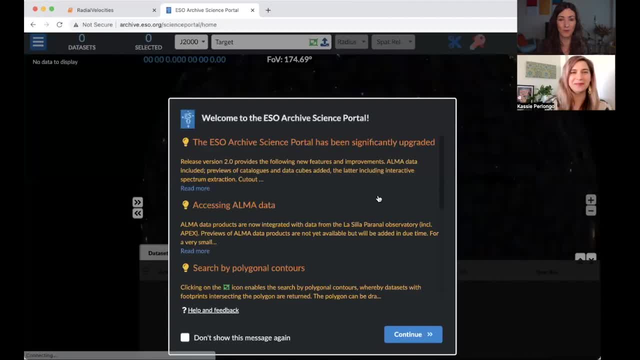 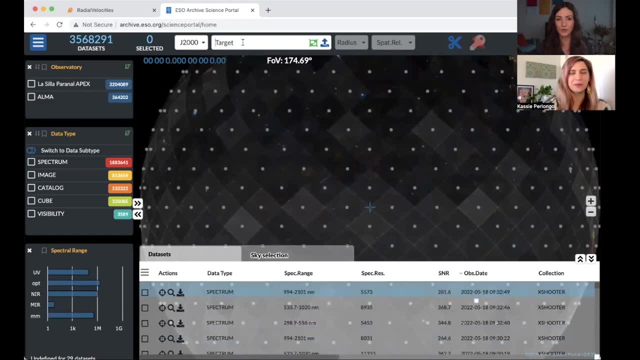 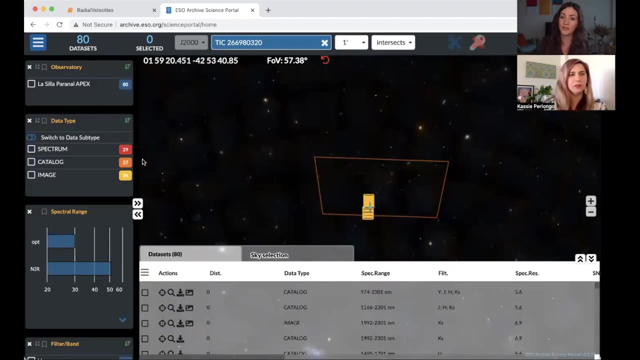 um good to know you can still look but it probably won't be in there um cool so you can take a tick id you can put it into the eso archive press enter and then it will tell you what data is available and the data we're interested in for the radial velocity observations 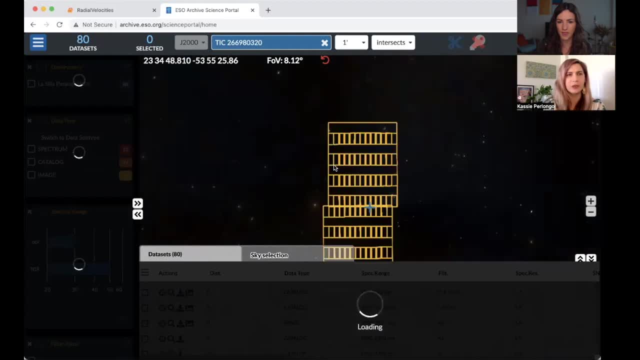 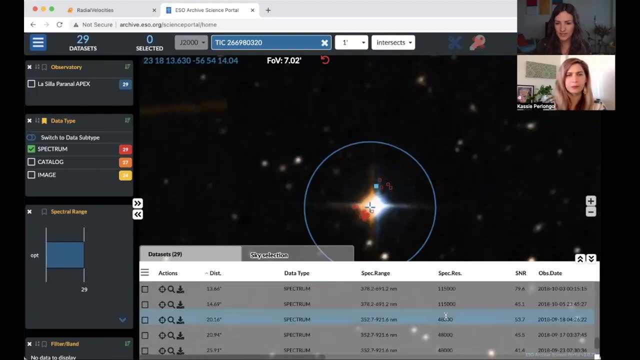 are the spectrums the spectrum website this is a cool website um and then you have this whole list um harps is always great if you see harps then 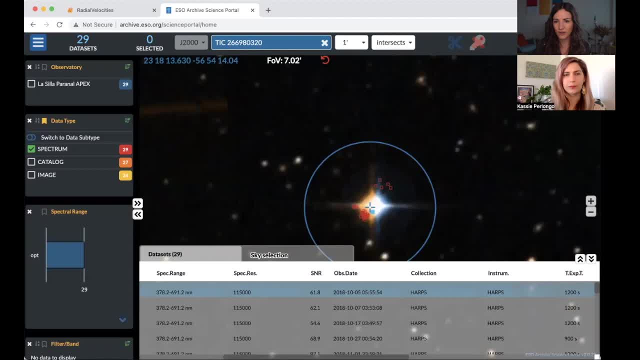 you should go for those um you can then download them by clicking in 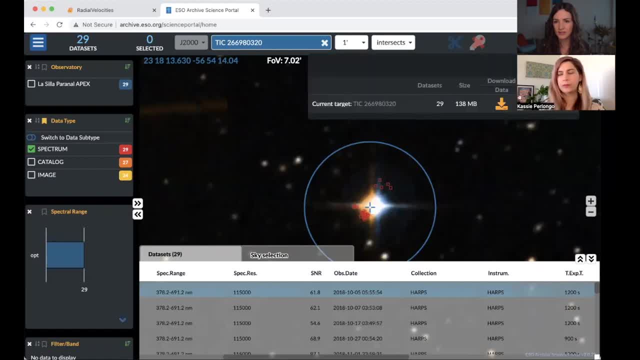 the top right hand corner on the download button what does that stand for sorry did i miss that oh sorry uh harps is an instrument on um a telescope so it's on a 3.6 meter telescope and it stands on a 3.6 meter telescope so it's on a 3.6 meter telescope so it's on a 3.6 meter telescope um 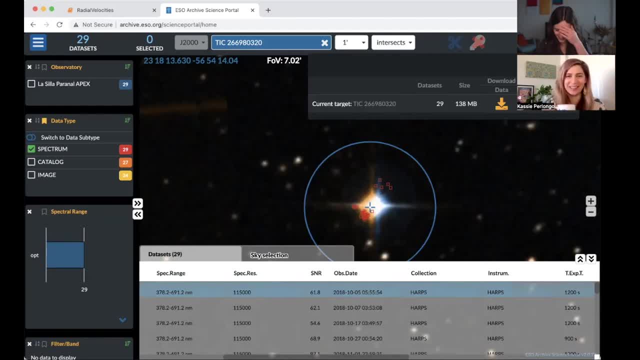 it's an instrument on a telescope that's as far as you need to know cassie thank you and good night 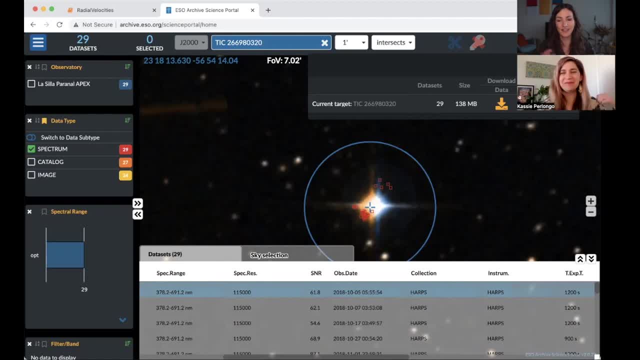 i should know this and i do know it i just it's not coming to me but i will you've got thesis brain still 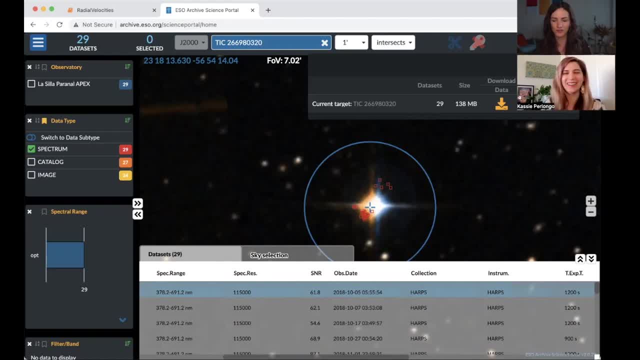 i'm pretty sure the piece stands for planet yeah high resolution 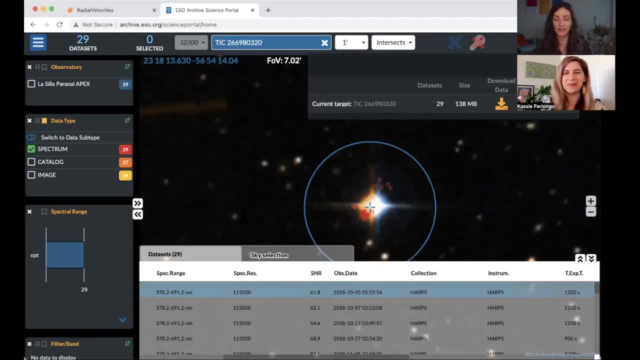 something whatever it's it's a it's a tool used to take spectra of stars and it's very good for finding 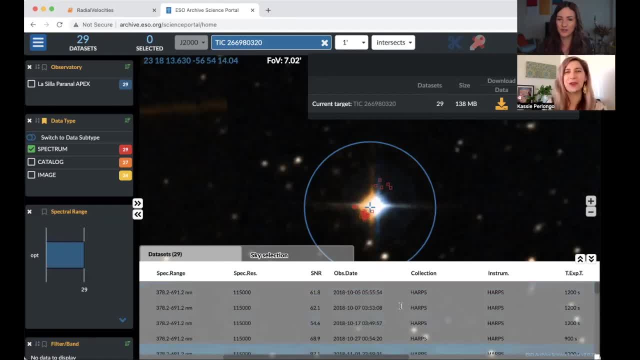 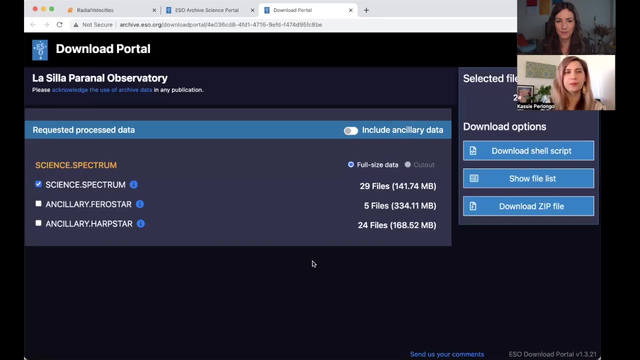 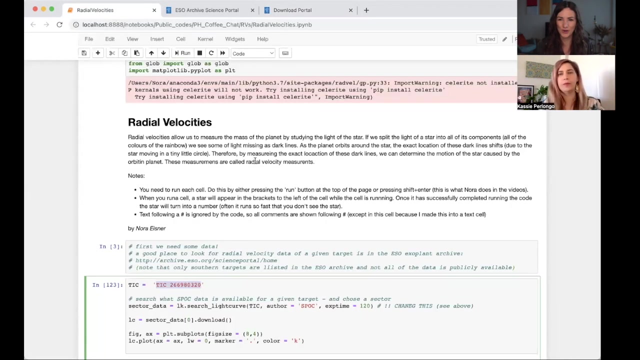 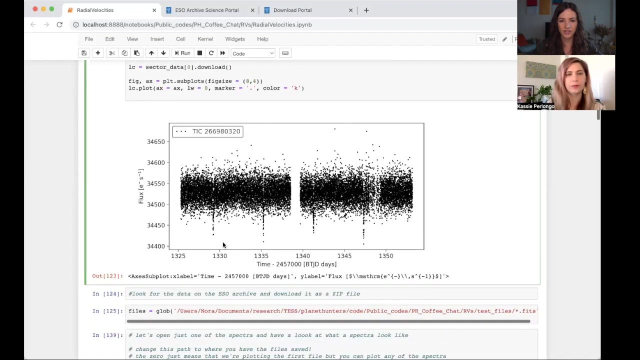 planets it's all we need to know right now that's great then you can go to a specific star look if there's any data and you can download it using the download dataset button in the top right hand corner and i also want to mention that if you do go onto that button you press on the the one that says data and then you get taken to this other page and you want to download the ancillary data as well so you just check that and then do downloads a file okay um so yeah if you want to use data you download it and store it on your computer and we'll go back to the notebook to see what we do with it then okay um so we're gonna look at just a random target this is the target this is a known planet that has been published i think it was found in test data um we're just downloading it here we can see that there's some nice transits in here i think it's a hot jupiter so So it's a large planet close to its host star, so with a short orbital period. 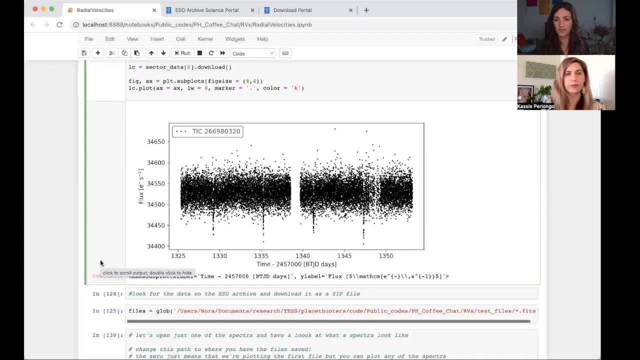 So these have larger radial velocity amplitudes. So these have larger signals, larger red and blue shifts. So they're easier to see in the RVs, which is why we're using it as an example today. Cool. 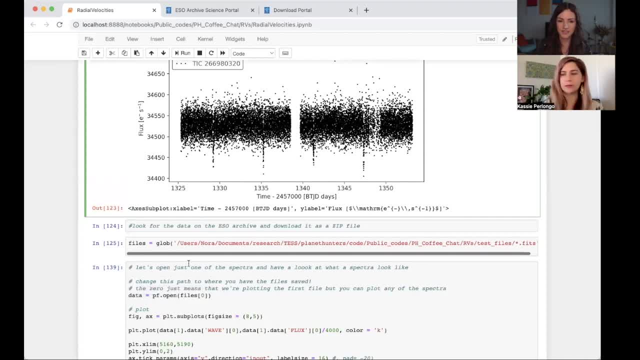 So you have to download the data and store it somewhere on your computer. And you can see I have a very messy computer. So I have a really long path to where that data now is. 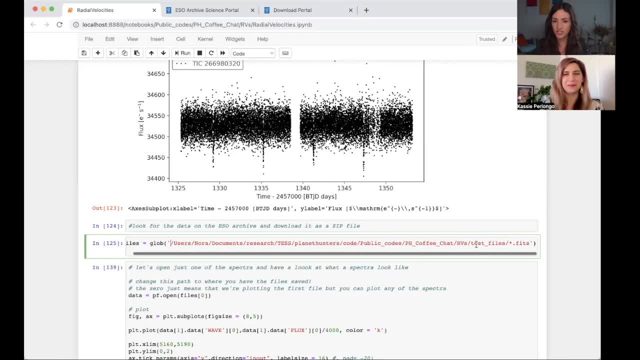 And so you have to change all of this to where you've stored the file on your computer for this code to run if you're running it at home. 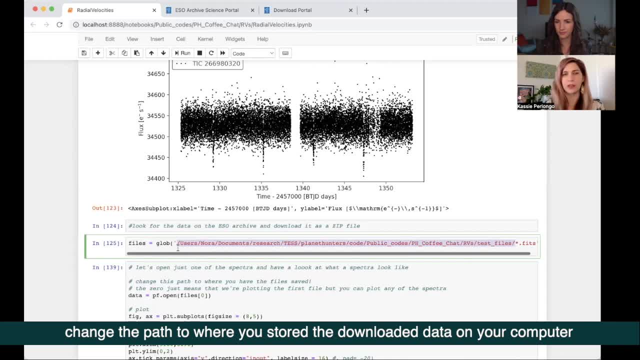 So yeah, do you put it on your desktop or something? Just make sure that it's got like the desktop and everything on there. Okay, got it. Exactly. 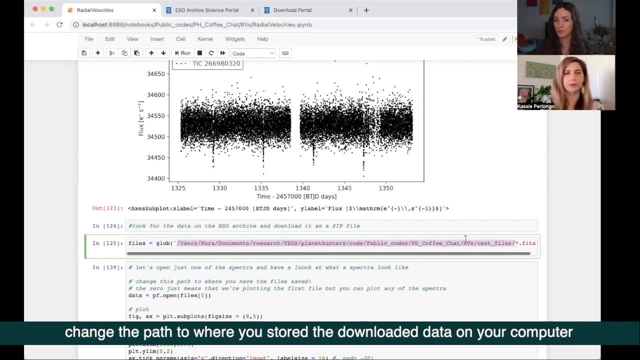 So for you, this might be users, Cassie, desktop. Then you've got it in a folder called test files or something along those lines. 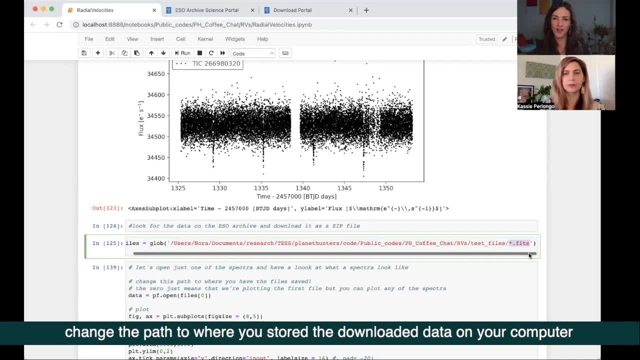 And then keep that star there. That star says, look at all of the files in this folder that end up in the desktop. Okay. So that's going to end in this. And it will then give you a nice list of all those files. Okay. Okay. That sounds good. Moving on. Cool. 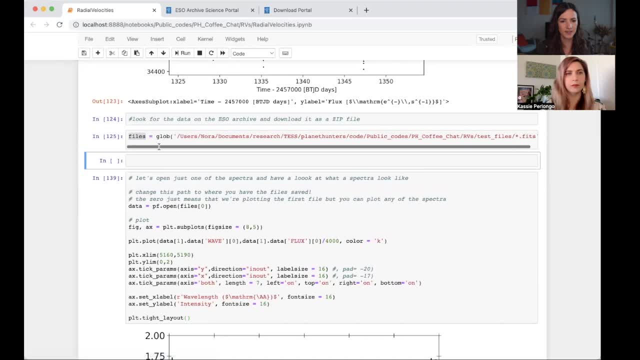 So what this now is, if we quickly just show this, if we insert a cell there, it's just a list of all of those files in there. So we can get rid of that again. We don't care about that list. All we need to know is that it is in there. Okay. Okay. 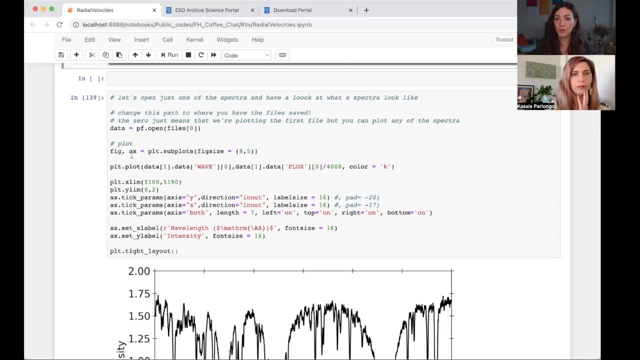 So we can make that a bit bigger. So what we're now doing is we're going to plot the data. We want to see. What this data looks like. 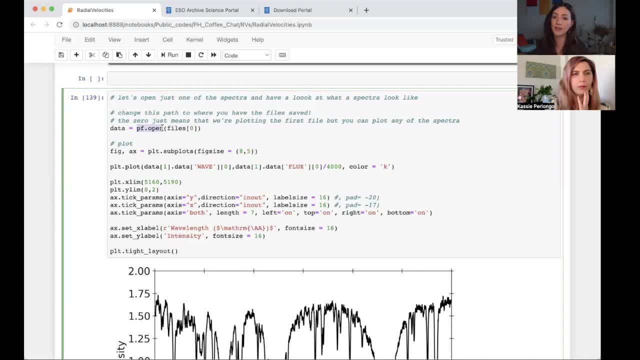 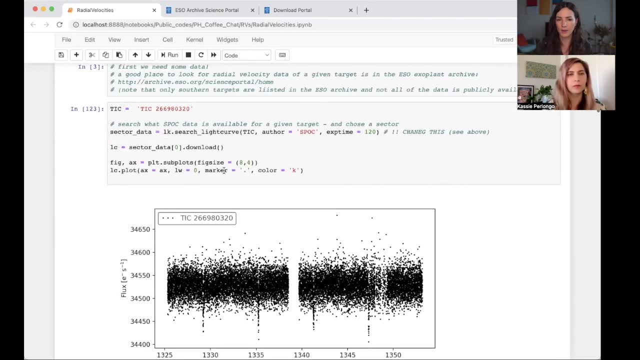 So we're opening this file using something called PF dot open. PF is just a module that we've imported already right at the top here, which can be used to open this type of file. 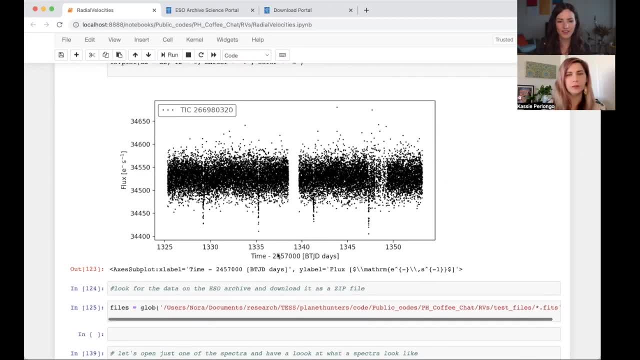 I should note we're using something called fits files. Fits files are quite can be quite confusing and tricky to use. What they essentially are is they are a file or a data file that have both data in it and information. So it has a lot of, it will have a column with. The it would just have part of that file, which would be all of the data. And part of that file will be information like who took the data. When was it taken? How long was that exposure time? Um, there's a lot of other information in there that will, we also want to extract, but just, just to keep that in mind, but we'll, we'll go through how to use it. Okay. 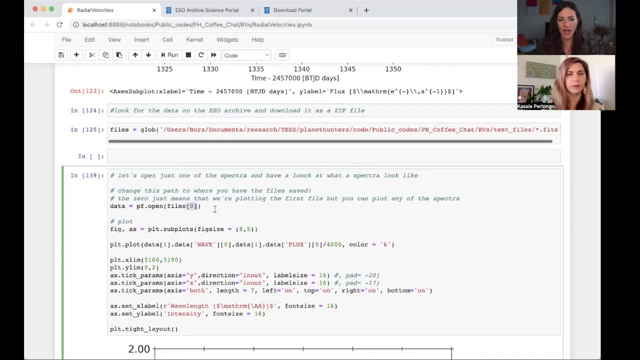 So we're just going to open one of these files. We're just taking the first one here and we're going to plot it and we're only going to show parts of it because I've okay. Excellent. 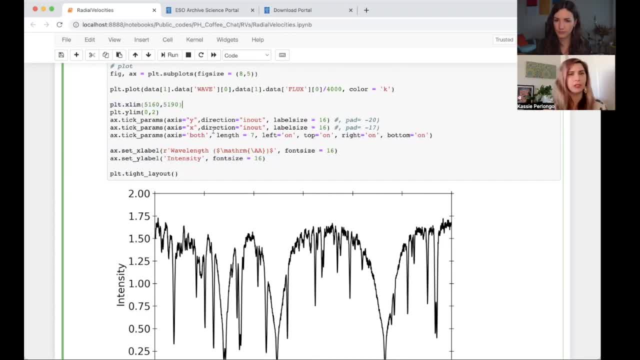 When you, when you plot it in, uh, at the beginning there, this will all happen automatically, right? There's no other things that you've put in that, uh, the citizen scientists have to also do, right? 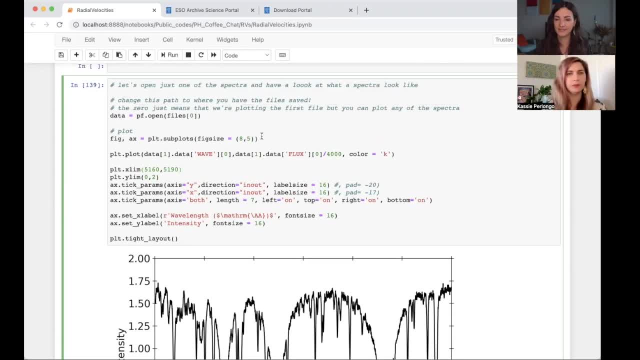 They can just, um, just change the path and then, oh, download some data to, um, uh, change the path and then this should all just work. Okay, cool. Okay. 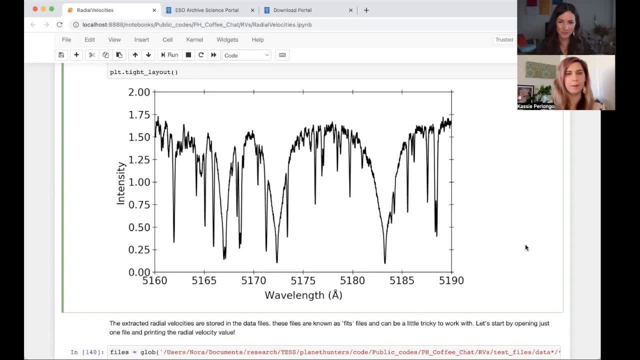 So this is an example of some of the data. So. What? 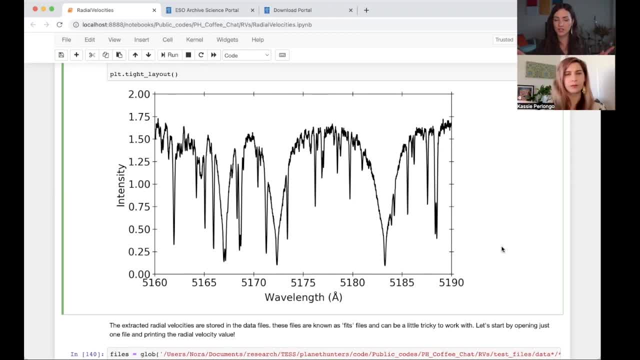 This is showing is it's showing you have the wavelength at the bottom and you have the intensity at the top. So you can see that this has a lot of different absorption lines. The, if there were no absorption lines, this was just light, just pure light that hasn't had any interference with it and the atmosphere in the way, then all of this would just be a straight line up here, but here we are seeing lots of different absorption lines and what we can see with this spectra in particular. 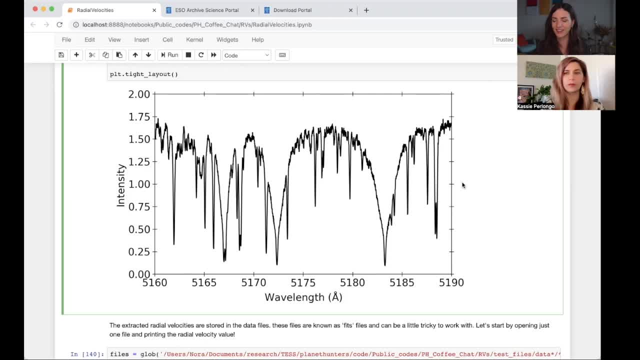 So I keep saying spectrum with this spectrum, spectra is plural spectrum is singular. I get it wrong every single time. Just bear with me. 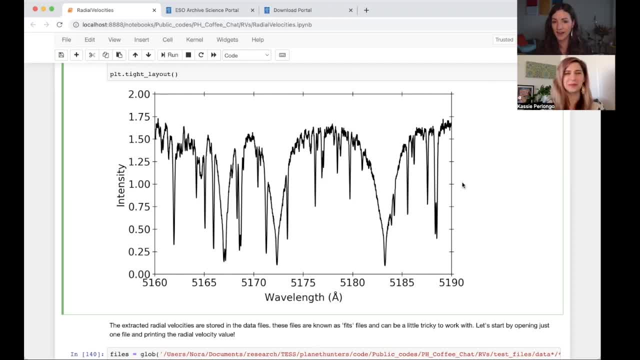 We can see these lines that these steps that we're seeing these lines, they're really clear and they are, um, they're, they're quite narrow. So this is a really good start to look at. We've got high, what we say, signal to noise. We have a lot of signal and not very much noise, um, not very much scatter. 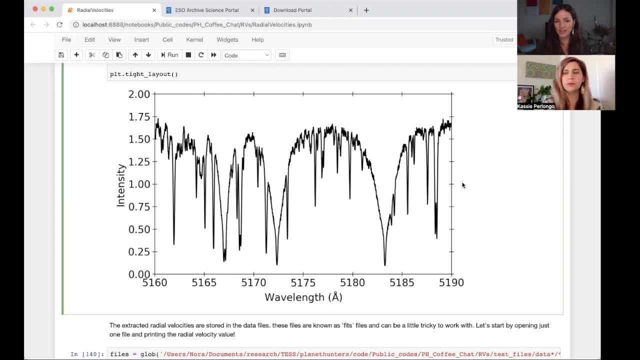 So this is a good start to do radio velocities with, um, if you can imagine if you have these lines smeared out, then it would be a lot harder to measure their exact location and we really need their exact location. 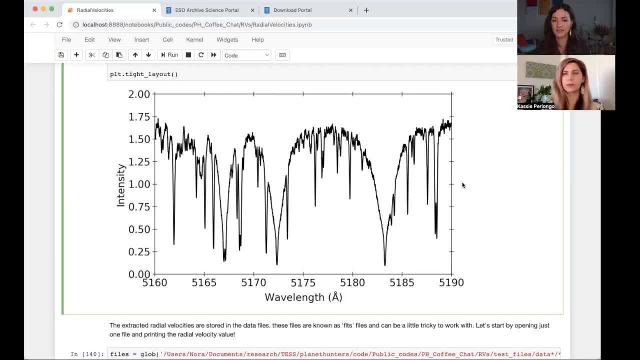 Um, because the stars wobble on such small scales that those exact locations really make a difference. Okay. 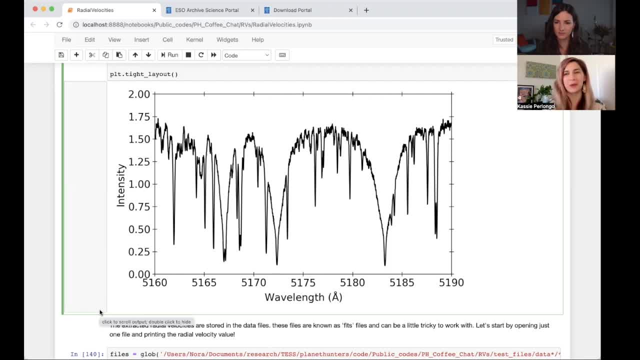 So this is not one that you could be off by a little bit and have the same thing. It could actually determine whether or not. Okay. 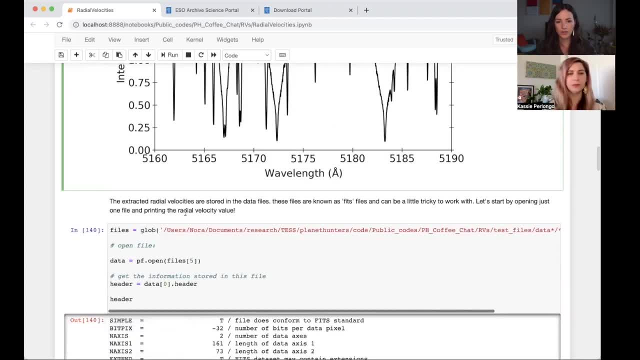 This needs to be very, very precise. Okay, cool. 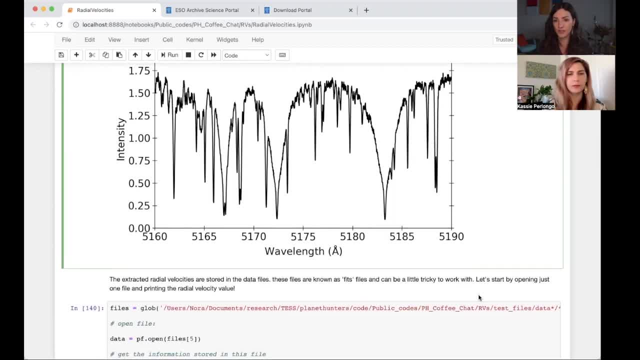 So that was just an example to show what, what one of these, um, spectrum look like spectrum spectrum. I'm not confused, which one's plural and which one, anyway, it doesn't matter. See doctors. They're just like us. I love it. I'm not a doctor yet. You might as well be at this point. 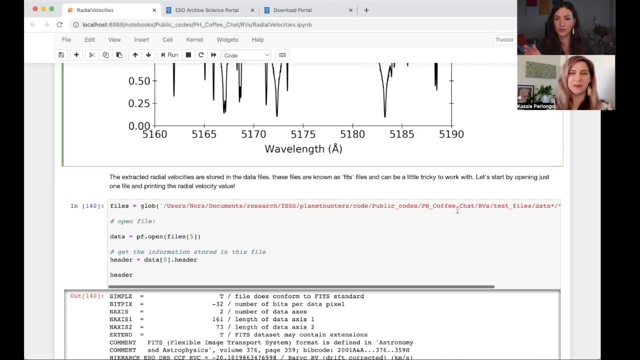 So we're now going to look at, so remember how I said you have to download both types of, we have to download the data and the ancillary data. So now we're going to use the. Yes. 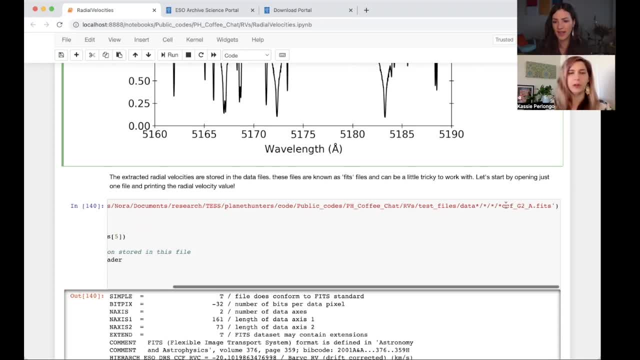 The ancillary data, which is also in that file that you have downloaded. And we want to use files that end in G two eight fits. Okay. 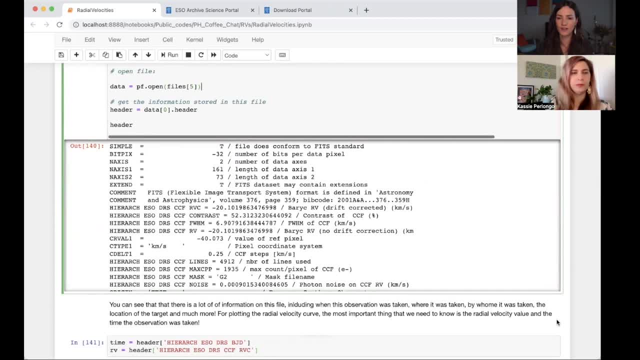 Um, and the reason why we want to use those files is because those files have the radio velocity, um, measurements already extracted. 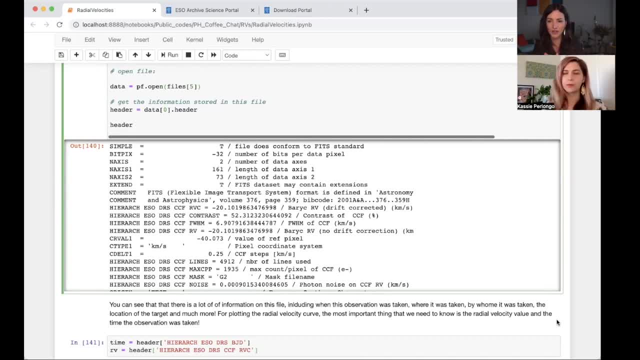 So those have those measurements extracted where it's telling us whether it's shifting slightly in one direction or slightly in the other direction compared to where we expect those lines to be. Right. Um, sorry. 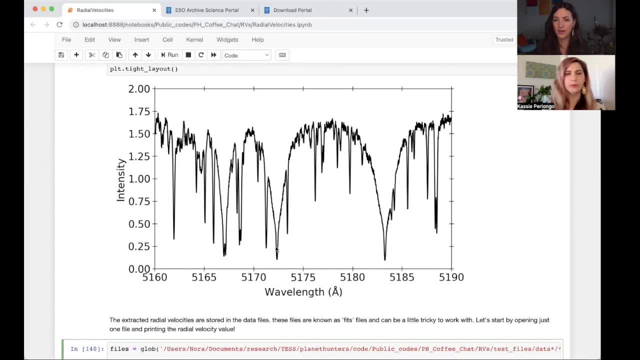 So what I didn't say actually before is that these, all these lines or these absorption lines. Also, if it's, if the object isn't moving are expected to happen at a certain, at a certain wavelength, we always expect, so we expect these to always look the same if the object isn't moving, so we can compare these to templates of what we expect the rest wavelength, the non-moving object wavelength to be, and that's how we get these radio velocities. Oh my gosh. Sorry, information. 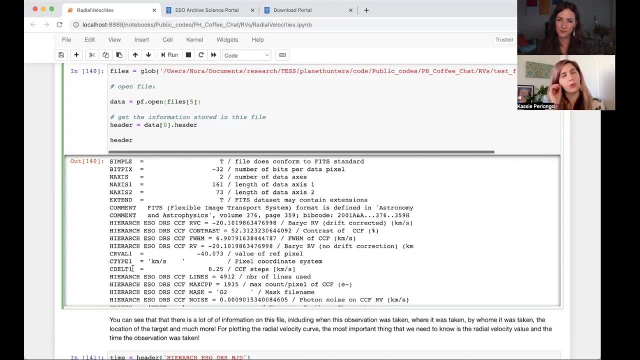 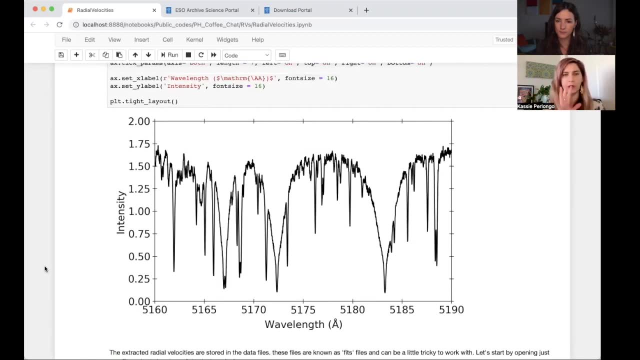 It's kind of intense because if you look at like those lines, can you, so when you just look at, can you go back up to the graph up above, can you tell by looking at that and where the wavelengths are, like, can you determine whether or not there's an atmosphere or you said, this is a hot Jupiter, like what can you determine from this? Just looking at the graph. Exactly. Maybe go over that once more. 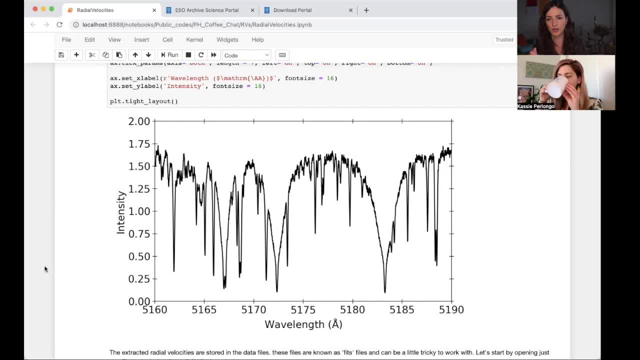 So this doesn't tell us anything about the planet. So we're not doing transmission spectroscopy. 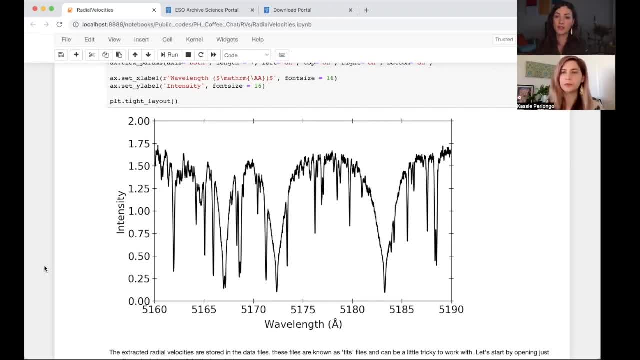 So transmission spectroscopy is where we look at the light passing through the star. What we're doing here is we're, this is only the light from the star. 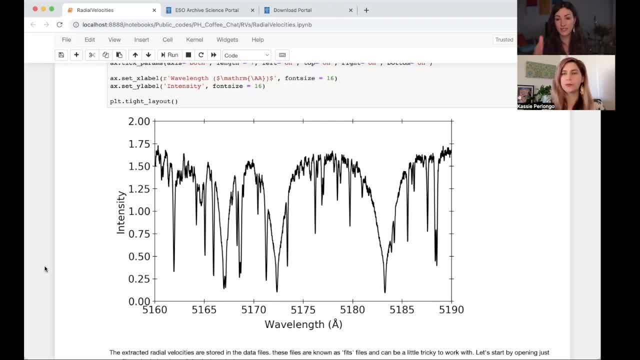 This is what we're just looking at. So this can tell us about what kind of star it is. Different types of stars have different absorption lines. So these lines will look different depending on how old the star is, how hot the star is, and all these other things. So, so this, this can tell us about what type of star it is, but not, this doesn't tell us anything about the planet yet. No planet. Okay. Got it. All right. Good thing to clarify though. Okay. So remember when I said that there's no planet? 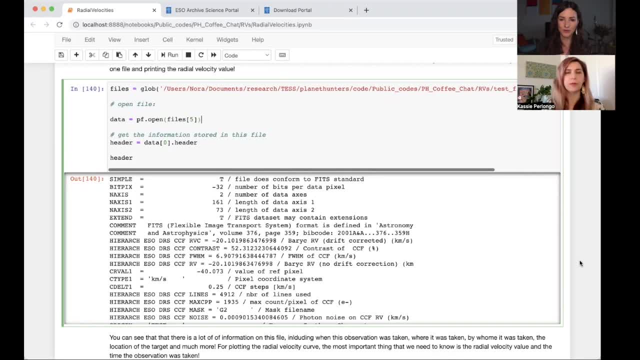 There are, these FITS files are very complicated and they have both data and they have lots of information. Here is an example of the lots of information. 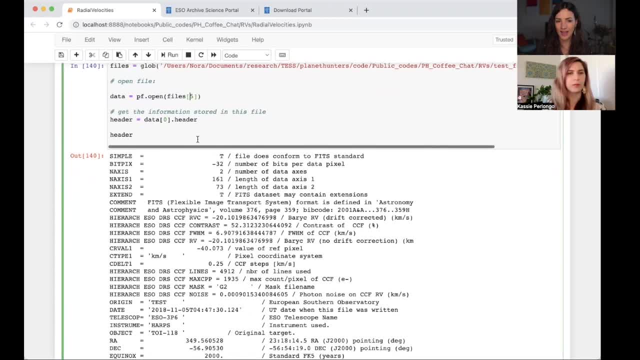 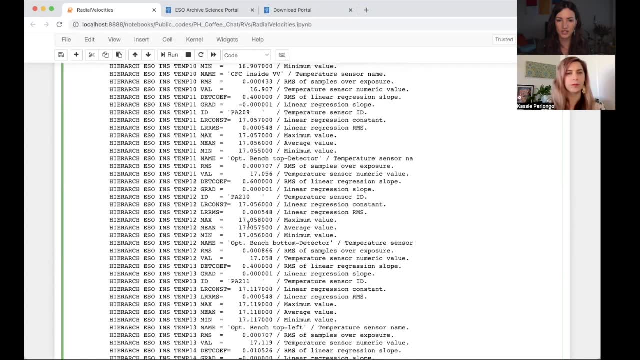 We are now opening one of these other files and we're printing, it's called the header where all this other information is stored. And you can see, this is just an absolutely endless list of just lots and lots of information that we don't really need to worry about. I'm going to make this small again. Okay. I'm gonna make that, collapse it again. 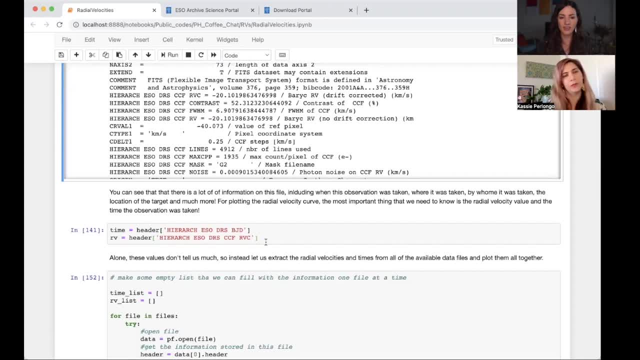 Um, the only two things we really care about for now are the. Um, time, which we can access using this command, this line of code here, and we want to know what the radio velocity observation is. So this is the CCF RBC is just what it's called. Okay. That's the code to put in. Yes. 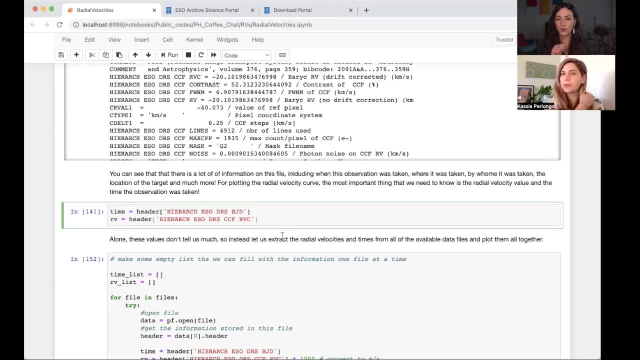 I should also mention, sorry, I should have actually said this before. So depending on what instrument this, the data comes from, even if it's from ESO, there are lots of different instruments in, in the ESO archive. 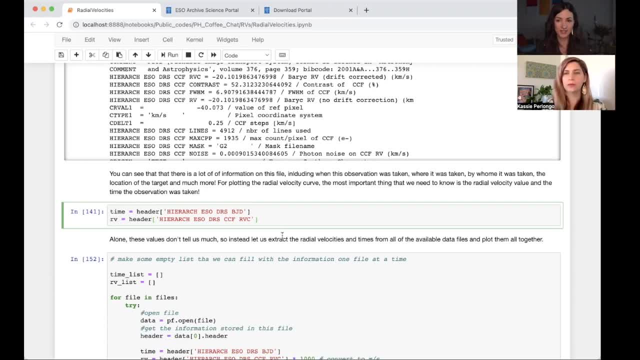 These commands will be slightly different. So I'm giving you the code to work with harps data and not with any other instrument. 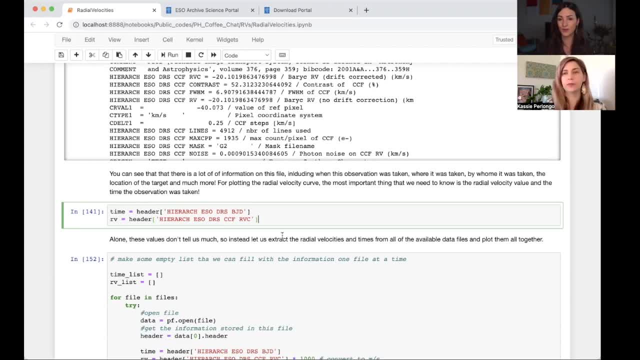 Um, but if you have questions about other instruments that you found data for, and you want to use, you can put a note in the chat and we'll have a look at it. Cool. Um, sidebar to remember. Yes. Yeah. Keep that in mind. Okay. 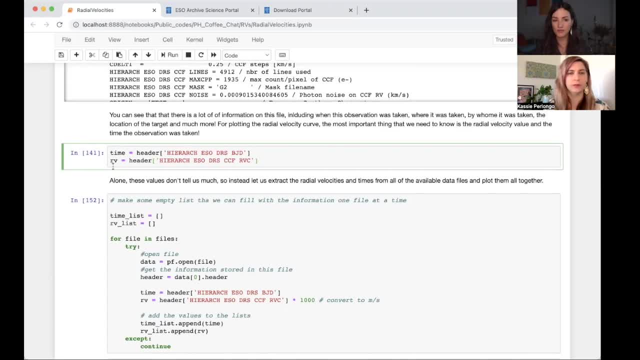 So we're going to open each file in turn and store this information of the time and the rate of velocity measurement, um, as a list, we want to have all this information together so that we can plot it because plotting is always useful. It. Allows us to determine properties. So that's what we're doing here. We are creating two empty lists. 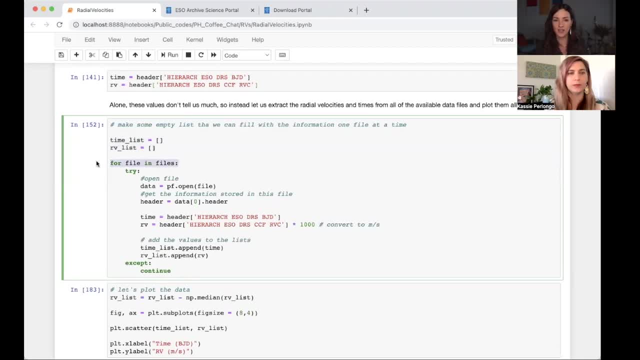 We are then looping through the file. So I'm saying for each file in turn, open it and tell me what the time and the rate of velocity measurement is that's down here and then just add it to that list added to this, what was an empty list at the start and at the end will be a full list. 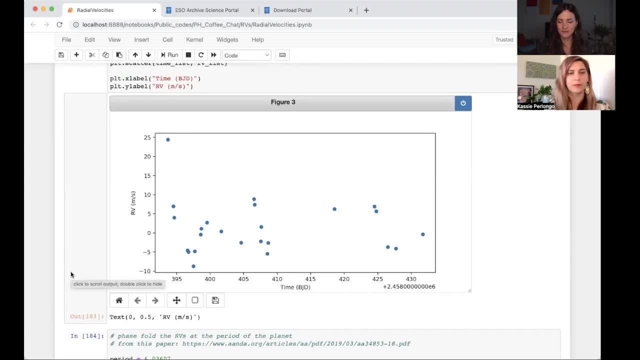 And then we have those two lists so we can plot them and you can see, this is just looks quite messy. This is just the rate of velocity in meters. Per second is how quickly it's moving in what direction versus the time. 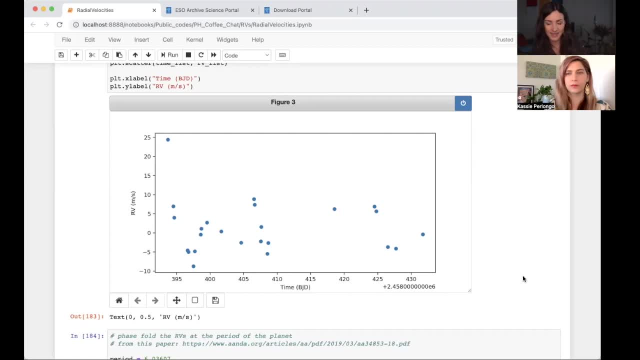 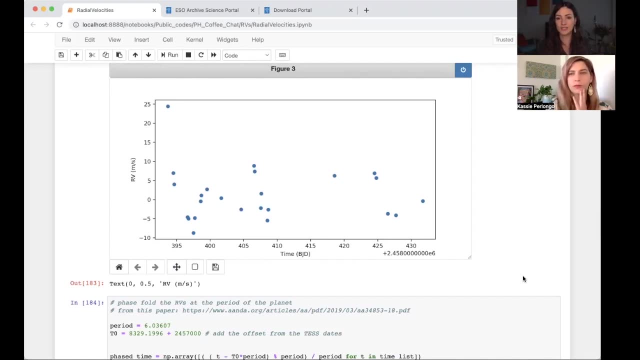 And this is, uh, I would say impossible to see whether there is a trend in that. So we'll scroll down. This was similar to what, when we looked at the, um, at the test data, often it was more difficult to see what was going on. 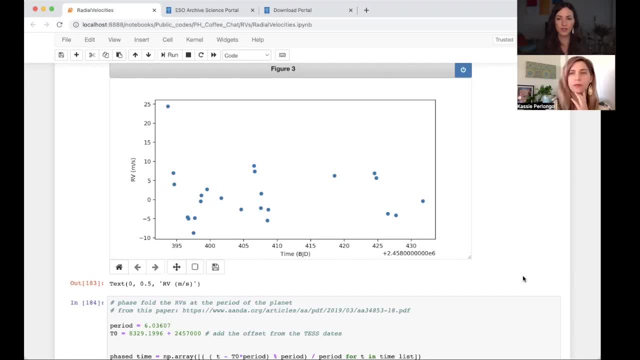 Um, when you just looked at the raw data and you actually wanted to face bold. 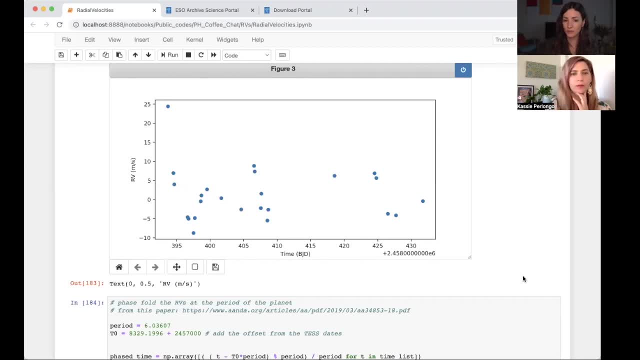 Um, so this is what we're going to do now. We already know the period because we saw the test light curve all the way at the start here. 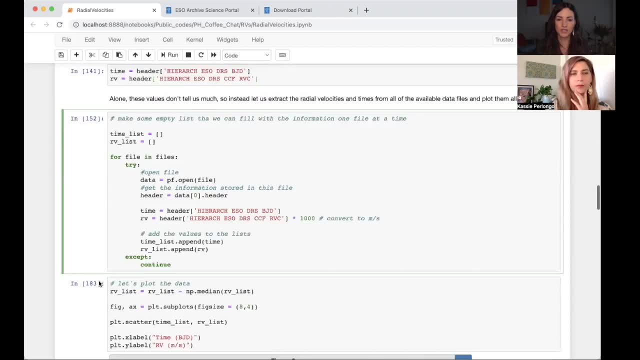 So we can extract the period from that. So we're going to do that. 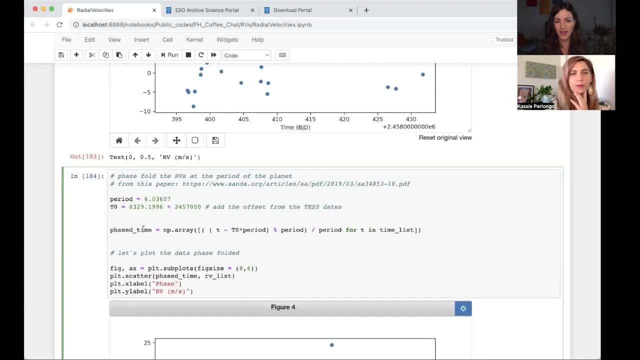 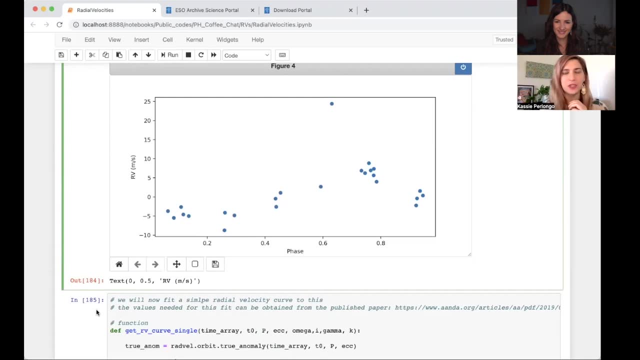 Um, and we've got the period, we've got the time we're going to face fold it, and then we're going to plot it. And quickly though, if you have any questions about that, and if you're like, I don't know what she's talking about with face folding, we have other episodes where Nora goes into it. Look at those or some of our earlier episodes as well. Yes. I'm face folding with RV data. 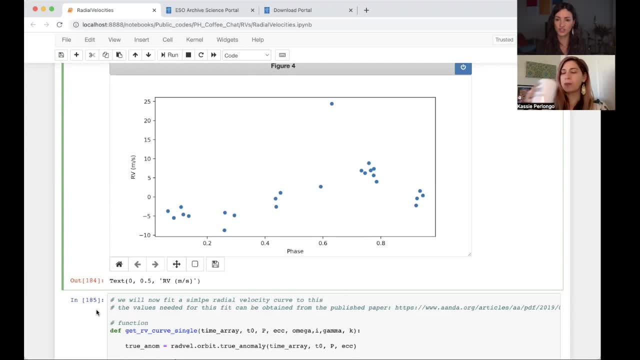 Creative velocity data is exactly the same as face folding with transit data. It's just folding, chopping things up and folding them on top of each other. Um, I have like this hand motion. I do whenever I show face folding like this chopping like this. 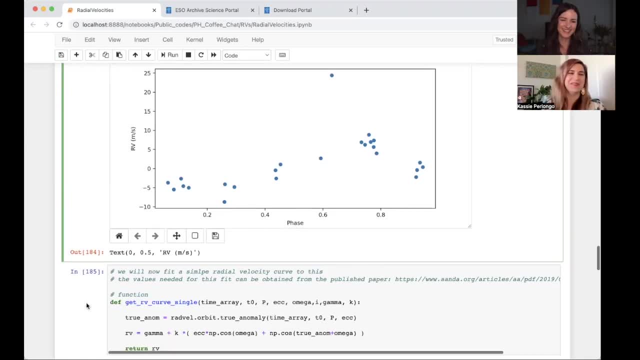 I like it. You know, just, I don't even need to say it anymore. I can just mark it out. 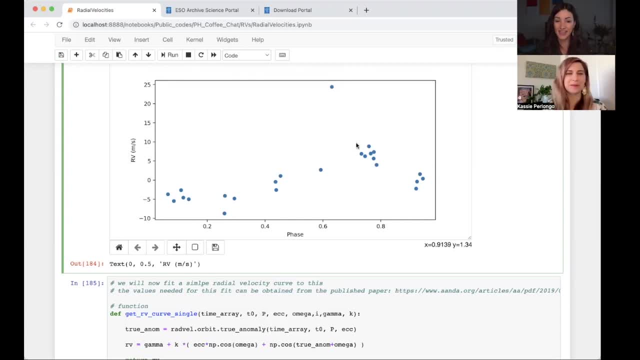 So this is the face forwarded data. So we can hopefully see that we're starting to see a slight curve. 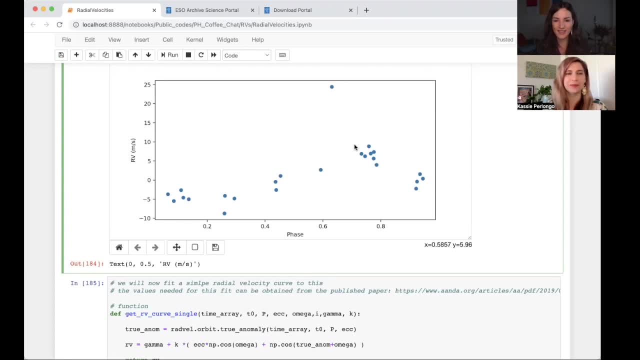 There is one data point all the way up here. We're not going to worry about that, but we're seeing a curve and you can see that sometimes this velocity. This emotion of it, the speed of this object of the star is positive. So it's, it's moving away from us and sometimes it's negative. So it's moving towards us so we can see it periodically goes from moving towards us to moving away from us. And that's because of this, um, large planet moving around it. Yeah. 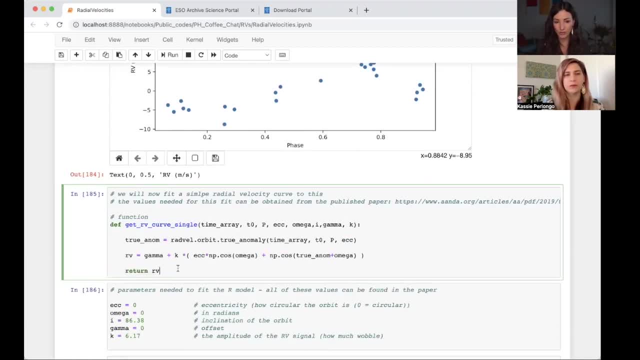 So to see this even more clearly, we can create a model for it. This is a very simple model. 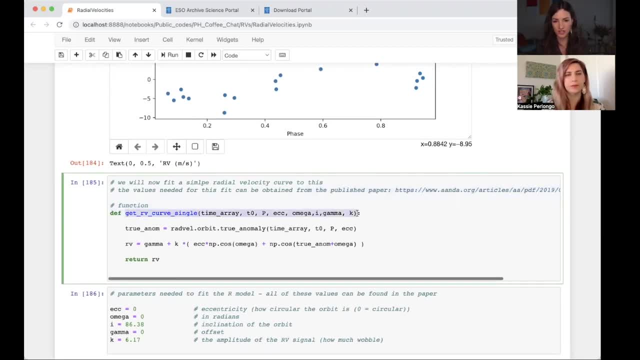 Um, you don't need to worry about the function itself. You just need to know that there is a function. 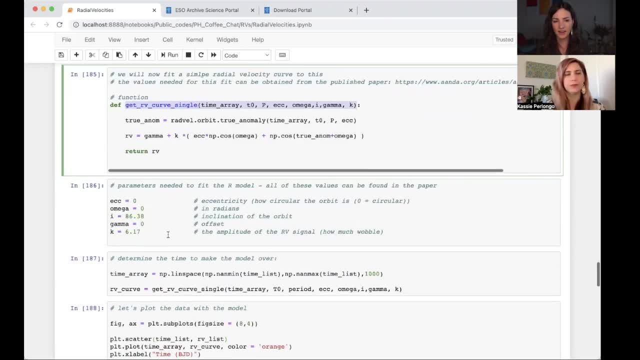 Um, this kind of this thing that you're seeing here, um, we have some parameters. You can usually, if it's a published system, you can get these from, from the publication. 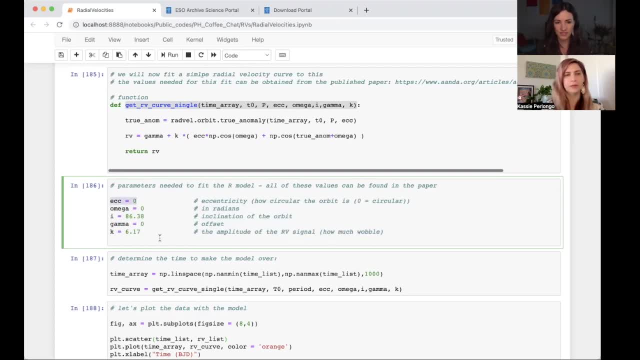 Um, so the eccentricity will just set to zero omega. We can also just set to zero inclination. 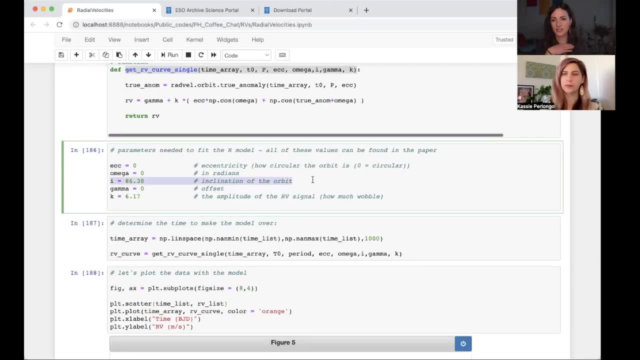 If we have a transiting planet, then we know that the inclination has to be close to, or exactly 90 degrees, because that's the inclination between. This is the star and we're over here, the observer, and this is the planet 90 degrees means. It's passing between us and the observer. 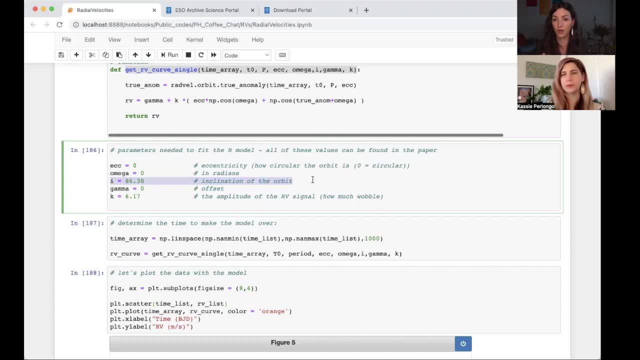 So we know if we are seeing this transit, it has to be nine or close to 90 degrees. Um, so this one is 86. So that's pretty close basically, so that we know that we're on the right track for it. Okay, exactly. 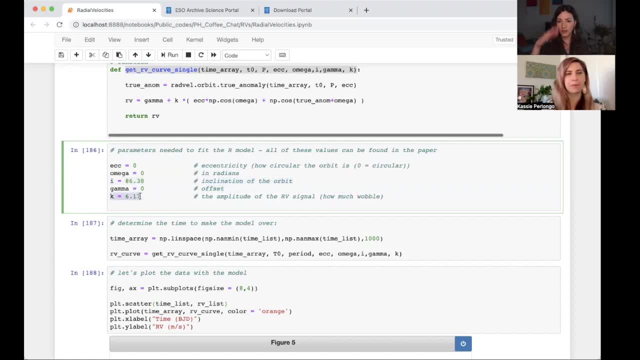 And K, this is the really important one. This is the amplitude of it. So how large that signal is. 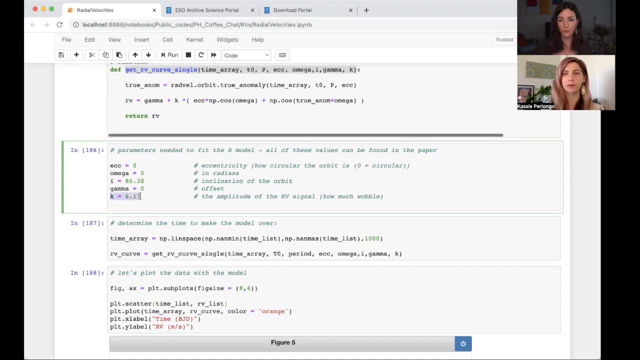 So that will then this, the amplitude is what we fit for is what we make the model with, but that will at the end to tell us how. Um, massive. How heavy this planet is, which is the information we want from this. So we can do that here. 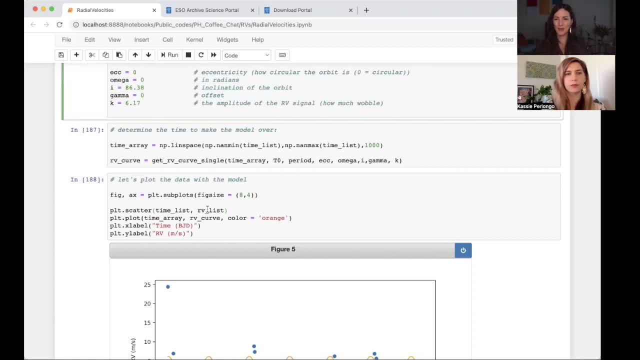 I've put in the values, which I know are correct from the paper that has been published. I'm just going to ask. 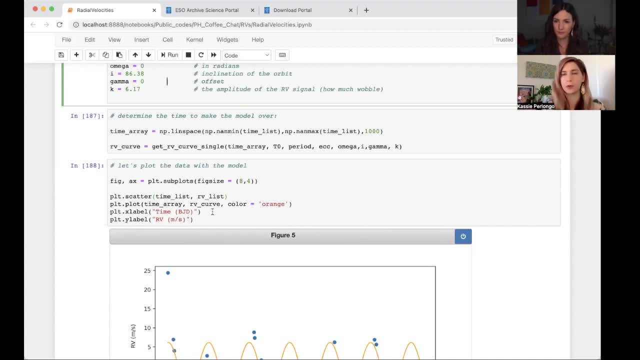 So once more, you got all those values from the paper that was published and you plotted those in. So if people wanted to do this for anything else, they would need to get it from the paper as well. Yeah. Get it for the paper is the easiest way of doing this. 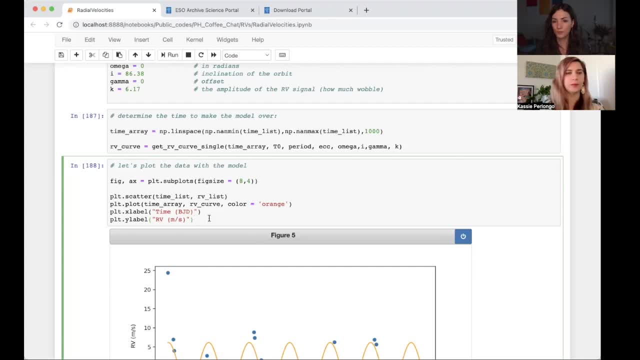 Okay. Um, or, or play around with the parameters. And see what you get. 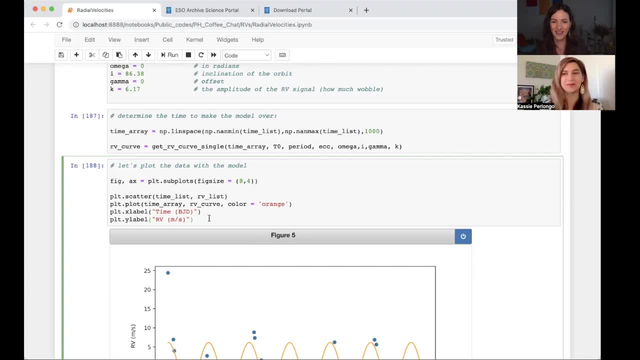 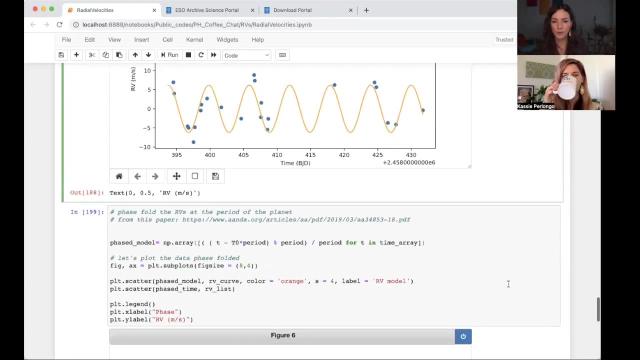 Yeah. Um, which is something to, um, okay, cool. So we have plotted, um, a line through it and we're starting to see that trend that we saw in the face forwarded model, but we can also face for that model. 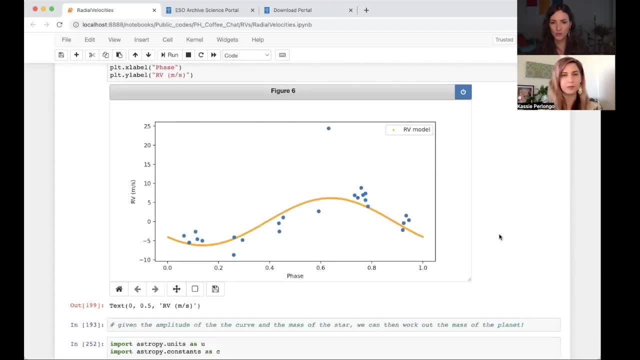 And here we have that line fit to the data and the outlier. We just ignore because that one is just whatever the one that's okay. Yeah. 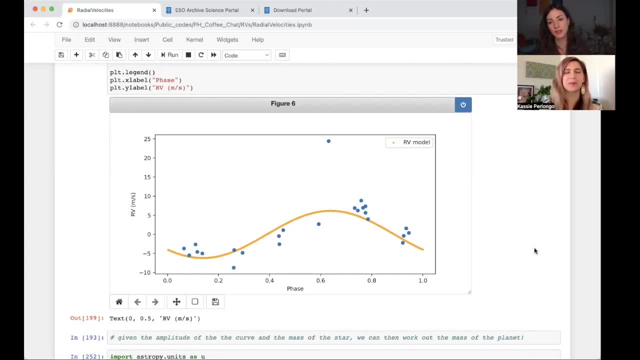 I'm going to assume that something went wrong with the radio velocity extraction. So this would be another case where you dig more into, into that giant header with lots of. Yeah. Lots and lots of information on it. 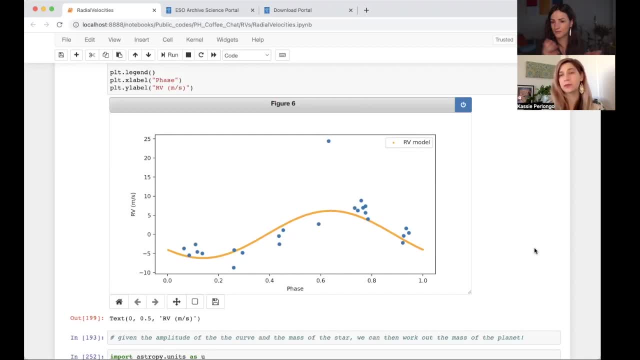 Maybe there was a cloud in the way. Um, maybe it was just taken at not favorable conditions. Um, there can be a number of reasons to why that point is wrong. 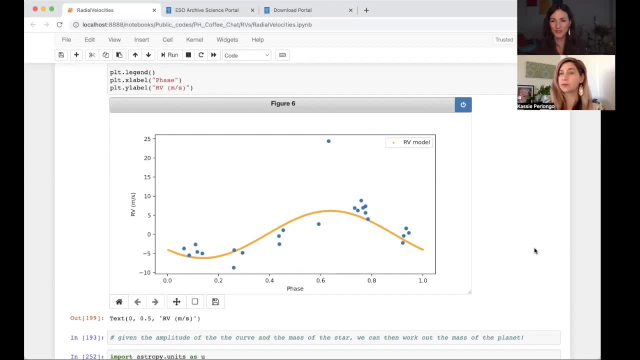 Maybe that point is correct. And it actually deserves further investigation, but for the, for the sake of today, I don't think we don't need to look into that. 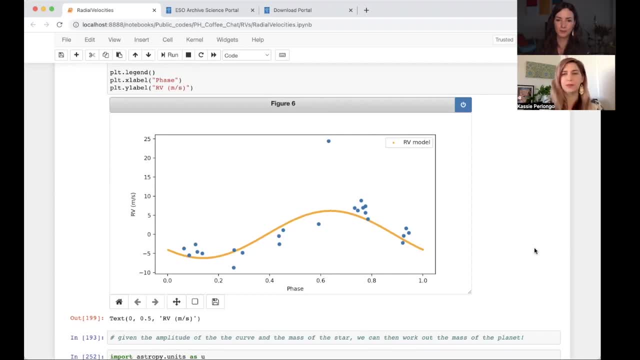 Um, we can assume that it's an outlier. Um, cool. Excellent. Okay. 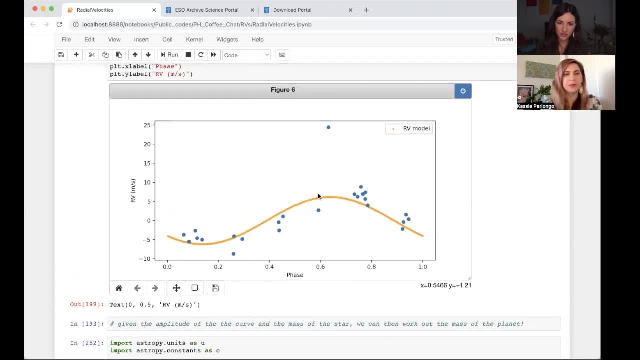 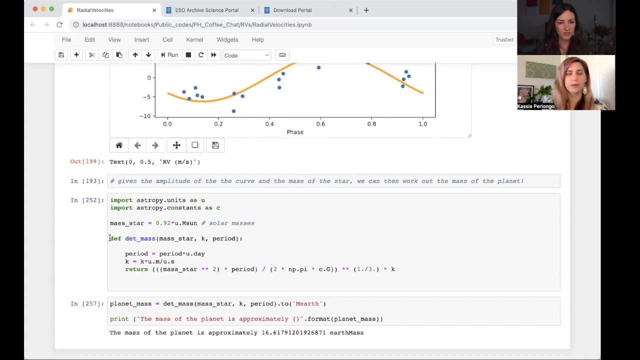 So given this, um, this is the last thing we'll do given this amplitude that we have given how large the signal is. Yeah. We can now determine. How heavy this planet is, how massive this planet is so we can do that here. It's with this function called to determine debt, underscore mass to determine the mass of the planet in order to determine the mass of the planet. 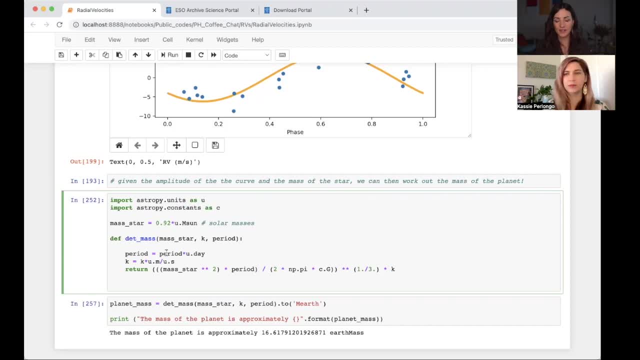 We do need to know the mass of the star, and we can get that information from, um, from ExoFOP. So we love ExoFOP. We use it for everything. ExoFOP is a great website. 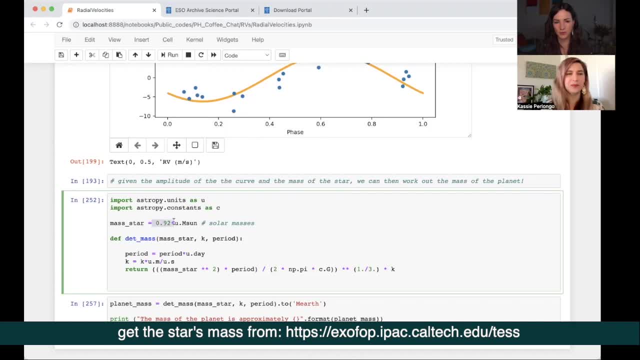 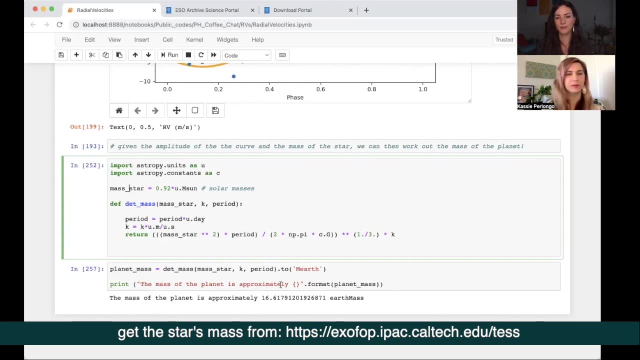 Yeah. So we can get that value from ExoFOP for this case. It's 0.9. Two, um, we just determined that here, and then we can run this function and that can tell us that this mass has an approximate, this planet can't speak. This planet has an approximate mass of 16.6. Um, times the mass of the eye. Yeah. Very exciting. Gosh. Okay. 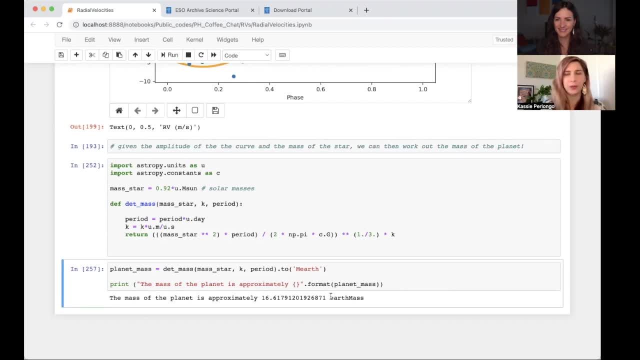 So there was a lot going on here, but you're going to upload the notebook so that people can follow it. Okay, cool. So what are going back through here? Um, because it was. 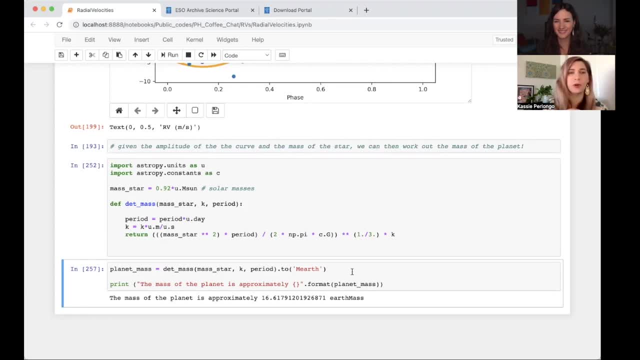 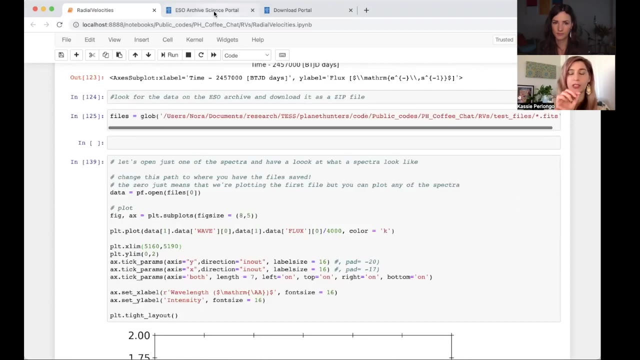 I, I'm going to have to go back and review this, to be honest with you as well. What are some of the main summary points that you want people to be aware of just so that while they're going through it, downloading the stuff from the, the ESO arch, uh, archive science portal, ticking that second box where they get the ancillary information. Yep. Uh, make sure it's the HARPS, the HARPS star. Okay. And, um, yeah, go ahead Nora. No, no, no. That was it. That was a good summary. Um, yeah. 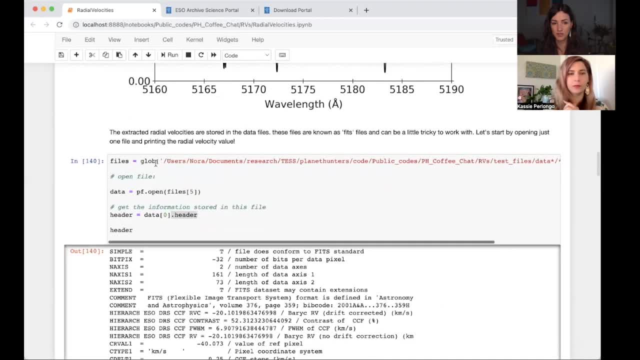 And then just make sure that wherever you download it onto your computer, the most important thing, because it works, this code won't run without that is that you point this path here needs to point to where you put it on your computer. Okay. Um, so if you put it, if you've downloaded it and it goes into your downloads folder, this will probably, if it were on your computer, Cassie, it would be users, Cassie downloads. Okay. And then everything after it makes sure, and then you've got like the forward slash data, um, and all of that, you want to have that in there. Yeah. So this would, for example, be downloads and then put it into a file called beta and you'll find it from there. Okay. That's good to know. 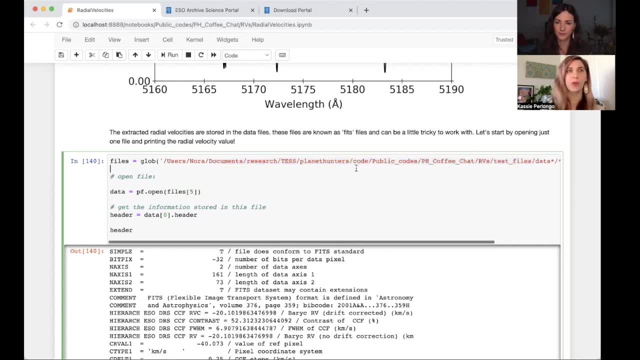 And then everything else you can look up from both either the paper or from ExoFOP, which is one of our favorites that we've gone to visit many, many times and otherwise just plug in, plug and play. It's a plug and play. 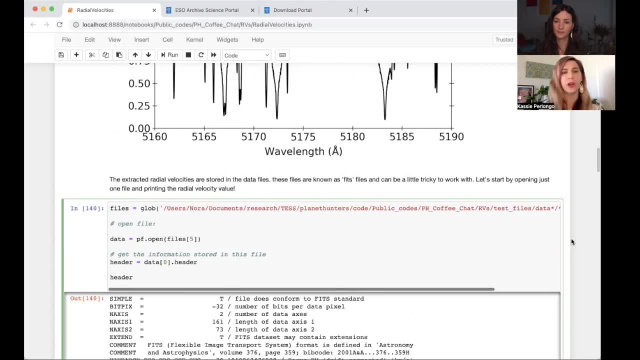 Look at, look at what Nora's already put together. Have a look through there. 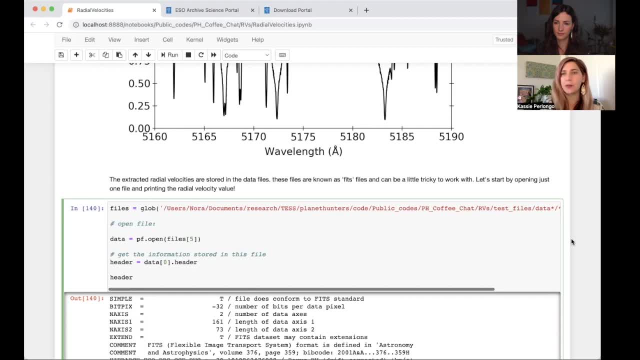 Um, is there. Maybe another TIC ID example that you could put, not right now, but maybe just to give the citizen science, uh, citizen scientists, um, an opportunity to go in and just try it on another TIC ID as well. 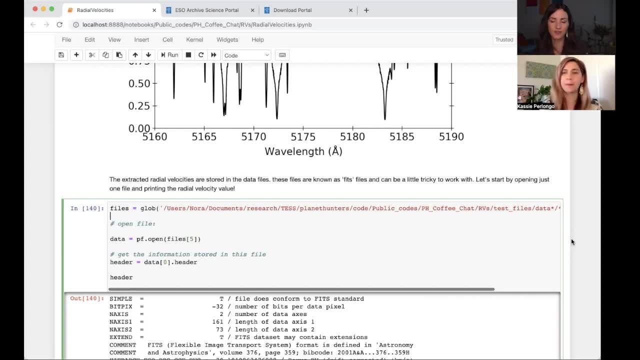 Um, yeah, you can try, um, my favorite TIC ID, TIC 55525572. Um, we'll, we'll do an episode where we go through the entirety of TIC 55525572, um, in a couple of weeks. 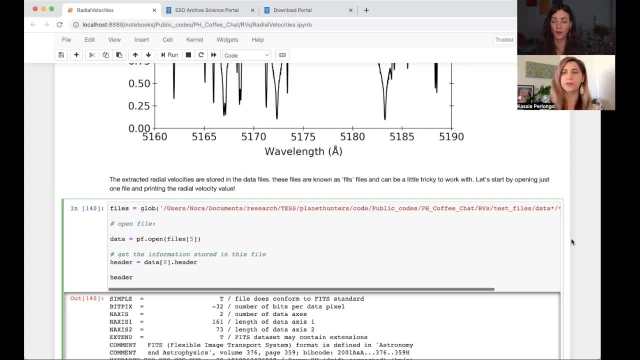 So we'll also, you can already play around with that and have a go, but we'll also show how we can get information from that. One, um, in the future episode. Excellent. 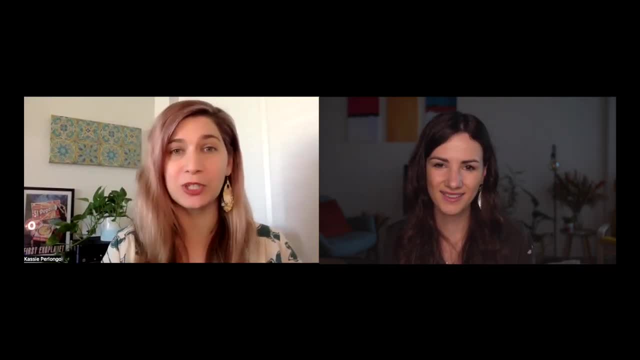 Was there anything else that you wanted to mention before we close out this episode for today? No, it's great to see you. It's been so long. It's good to see everyone. Good to see everyone. 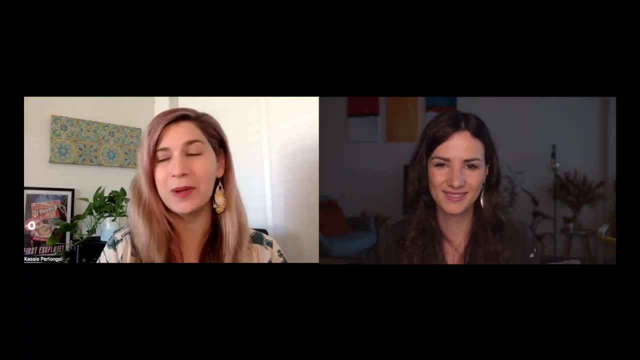 So, and I hope you forgive us for being off air for a while, but it was all for a good cause in the name of science, Nora getting her, uh, doctoral degree. 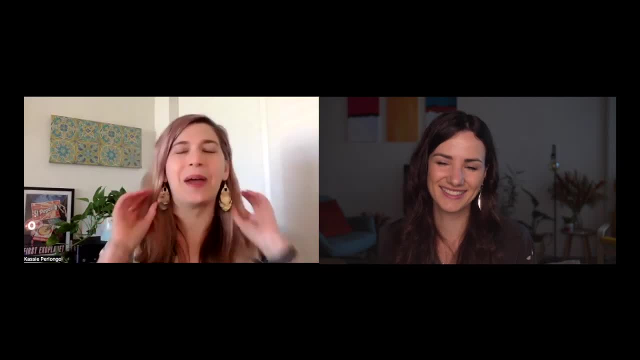 I mean, that's kind of a big deal anyway. Um, but yeah. Okay. 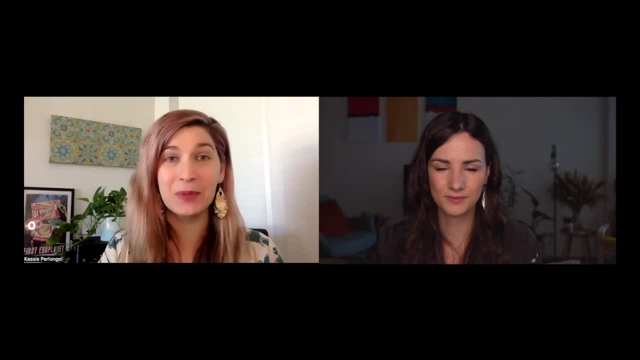 Well, thank you very much for joining us and, uh, Nora, I guess I will see you next week. 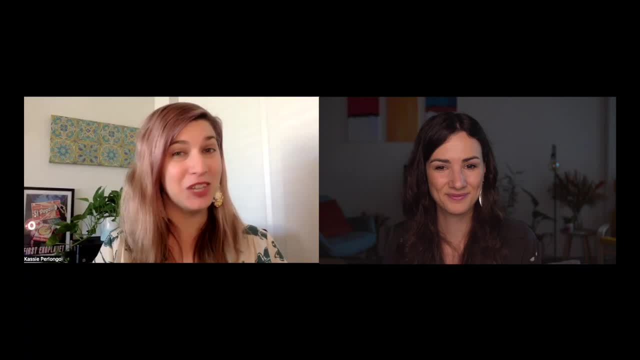 We're going to dive into astro seismology. I think that's what it's called. Star quakes. That's very exciting. I can't wait to talk about that. Um, and then we will see you guys then. So see you next week. Good to see Nora. Good to see you. Bye. Bye. Bye. 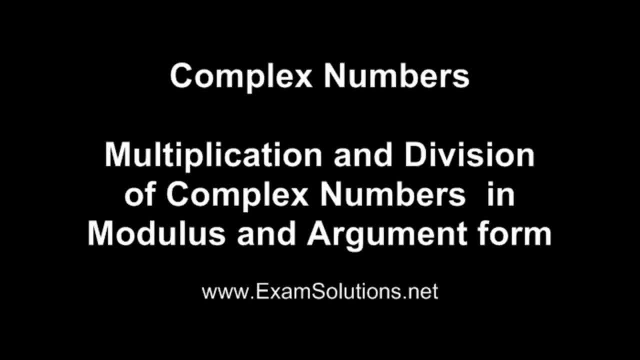 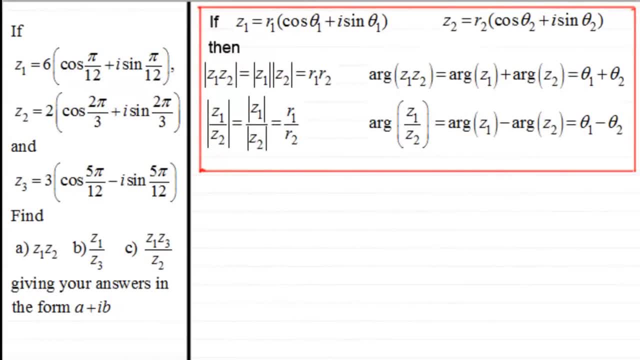 Hi, welcome to this tutorial, where I'm assuming that you're familiar with this result that concerns the modulus and argument of two complex numbers, say Z1, Z2, where you multiply them and where you divide them. If you're unsure of this result, you can always check out this. 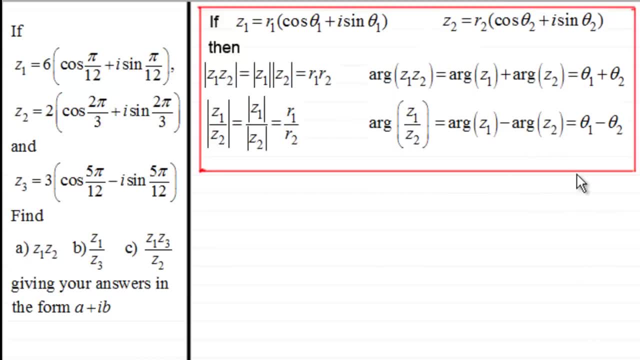 link here and it will run through the proof of these results. But what I want to do here in this video is just give you three questions to try. I've selected these questions because I feel that they reflect all the properties that you need to know essentially about using. 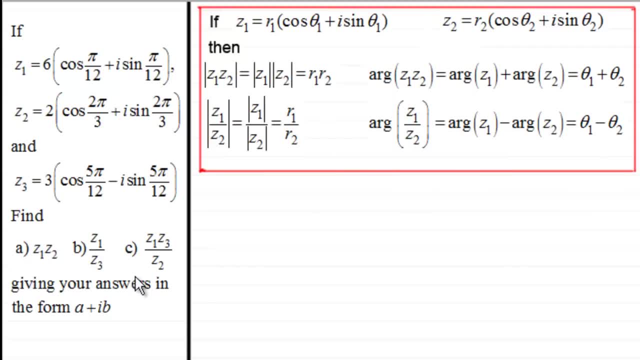 this result, So do have a go at this. You might like to just pause the video, come back when ready and you can check your answers. Or if you want to select any one of these solutions, just click on the buttons down here and it will take you to that work solution. 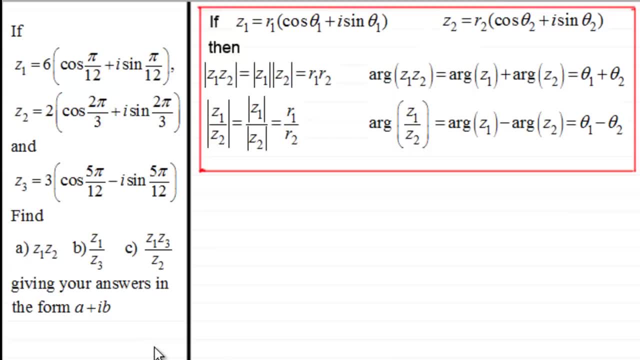 Okay, well, I'll give you a few moments anyway, just to pause the video and then select which question you want. Now for the solution of A. what we've got then is that Z1 multiplied by Z2, if we're going to put this in mod-arg form, then the modulus of Z1 times Z2 is given by this result. 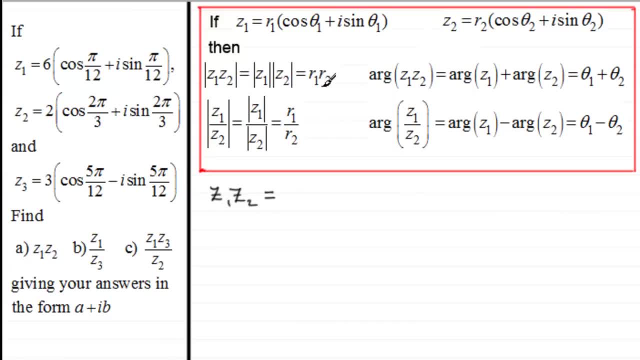 It's the product of the moduli of each of the complex numbers Z1 and Z2.. So that's going to be 6 times 2.. I know that's going to be 12, but I'll just put it in as 6 times 2 for. 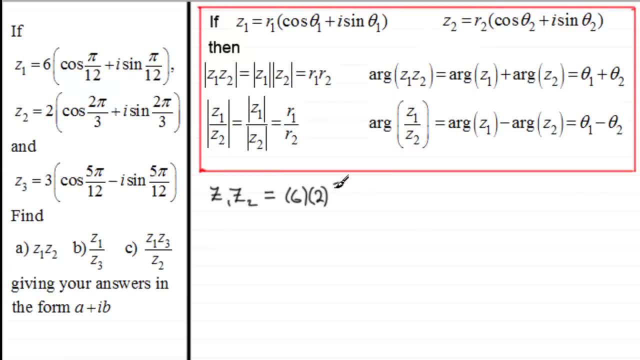 the time being, And then we multiply this by the cosine, or cos for short of the arg. So that's going to be pi upon 12 plus 2 thirds pi. So we'll have that then as pi upon 12 plus 2 thirds pi.